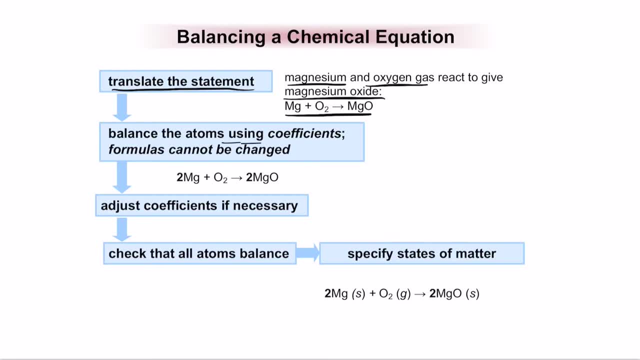 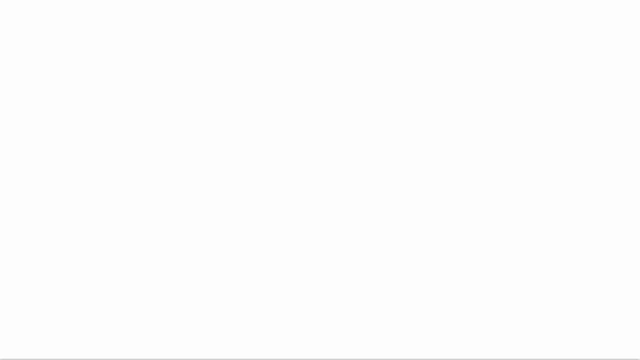 balance the atoms using coefficients and formulas that cannot be changed. so let's take a simple example of this. so we have converted the equation: magnesium plus oxygen gives magnesium oxide. now we have to add coefficients in such a way that we balance the elements on both sides. notice that. 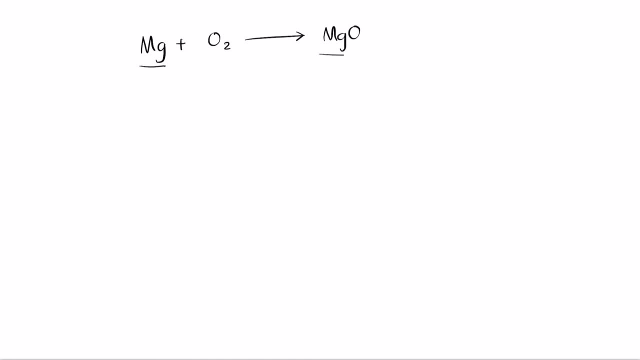 there is one magnesium and one magnesium, so we don't need to balance magnesium. next, there are two oxygen on this side and there's only one oxygen on this side, so now add two oxygens on the right side without changing the formula. so two magnesium oxides now, once you put two magnesium. 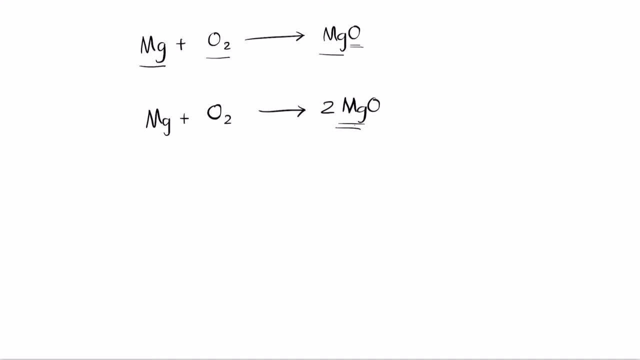 two. there magnesium became unbalanced because now there are two magnesium on the right side but only one magnesium on the left side. so now add two to the magnesium here, so two magnesium plus oxygen plus gives two m0. so check to see that all of them are the least multiples possible. 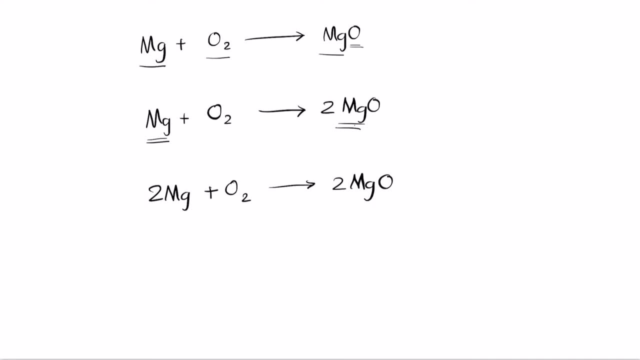 so if you have a common multiple, cancel the common multiple and write down the final equation. so now notice that there is two magnesium. so let me write it in different colors and let's say magnesium is the one in red color. so there are two magnesium atoms, one oxygen and there is 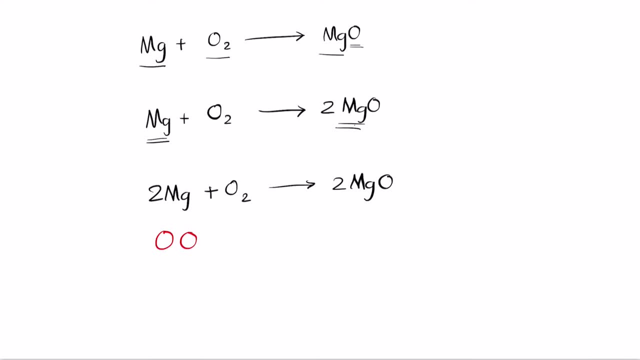 two. let's say oxygen is the one in blue. now you have magnesium oxide on the other side. so you have one red and one blue, and again you have one red and one blue. so this is the idea behind the balancing: notice that now on both sides there are two magnesium, two oxygens and two magnesium and two. 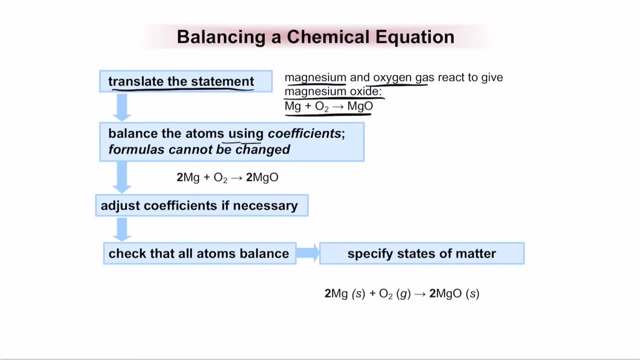 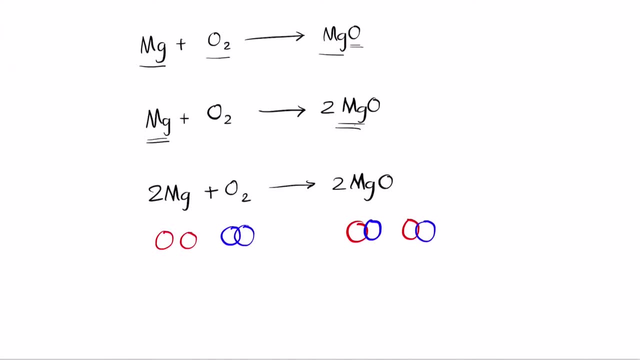 oxygens. so this is how we balance the equations, so balance the atoms and then finally adjust the coefficients, finally check the atoms, balance and specify the states of matter. here, how do you specify the states of matter? magnesium is a solid, oxygen is a gas and magnesium oxide is a solid. so with this, this, 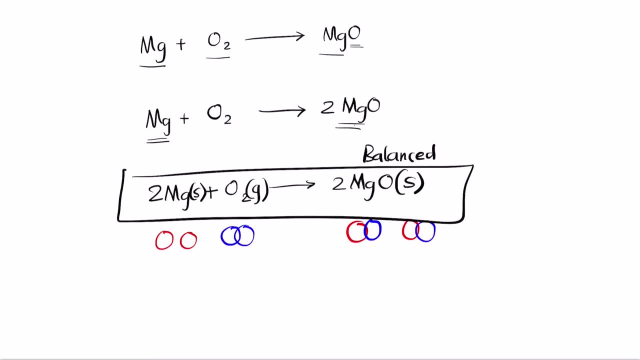 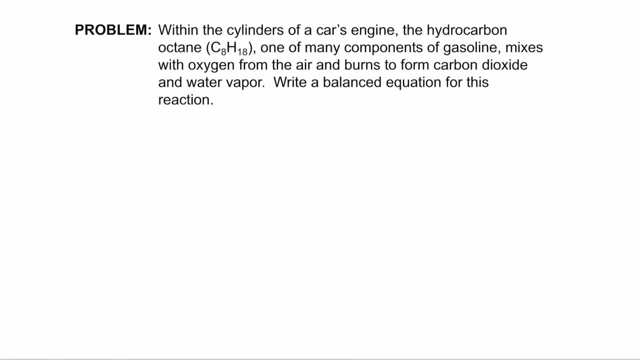 becomes the balanced equation. so this becomes the balanced equation. so let's take an example here. so within the cylinder of a cars engine, the hydrocarbon c8 h18, One of the many components of gasoline, mixes with oxygen from the air and burns to form carbon dioxide and water vapor. 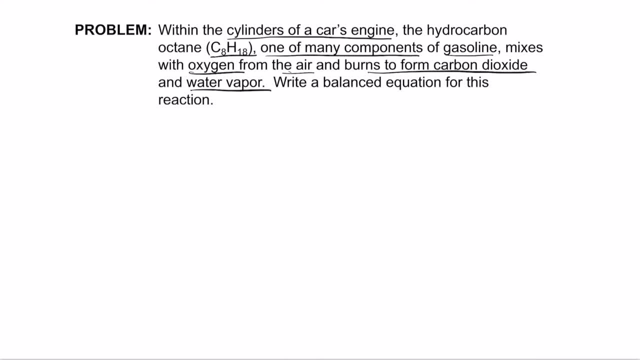 So write a balanced equation for this. So first let's try and translate the reaction here. So the reaction here is octane, mixing with oxygen to form air from the air and burns to form carbon dioxide and water vapor. So the octane is C8H18 plus oxygen in the air combines to form carbon dioxide, CO2, plus water vapor, H2O. 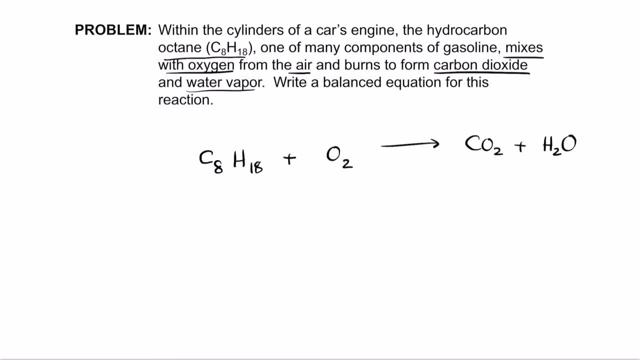 So the first thing we want to balance is look for each and every single element and try to balance one element by one element. Now let's look at the start. There is 8 carbon here. There is only 1 carbon on the other side. 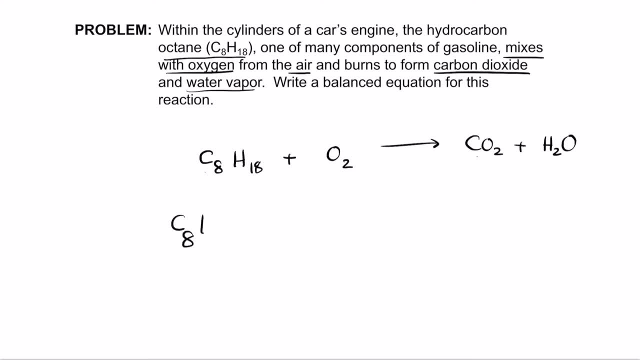 So that add 8 to the other side, So you have C8H18. Plus CO2 gives. So we are balancing 8 here. So 8 CO2 plus H2O. Now we have balanced 8 carbons. Now look at the oxygens. 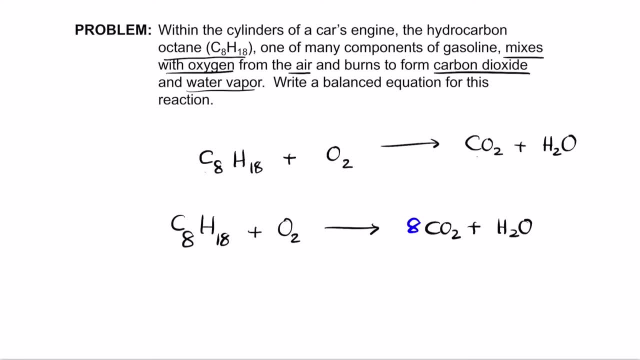 There is 8 times the oxygen, So that is 16 plus 1.. Right now let's look at hydrogen, The next one we want to balance on the right side, So don't worry about the rest of the part. There is 18 hydrogen. 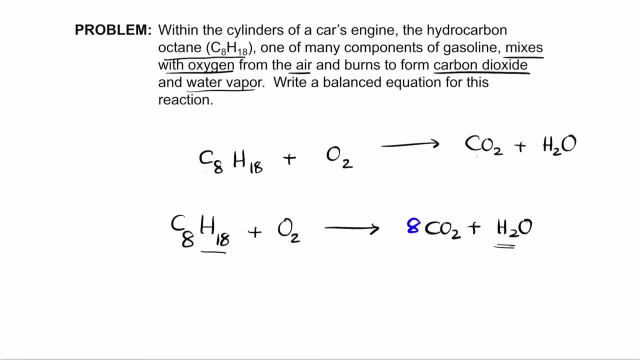 On this side there is only 2 hydrogens, So we have to add Multiply 9 to that So we get C8H18 plus CO2, gives 8 CO2 plus 9 H2O. So these are the multiples that we are using now. 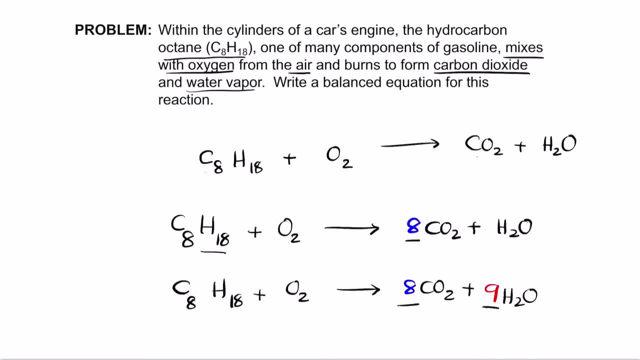 Now check for the balance on each side. So 8 carbons and 8 carbons are balanced- 16. So 18 hydrogens and 18 hydrogens are balanced. The last one that is unbalanced is oxygen. Notice that on the right side. 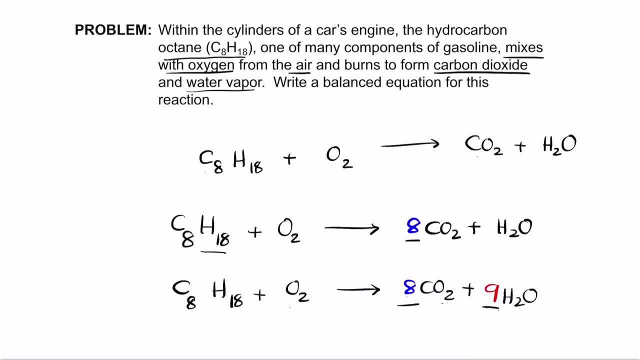 We have 8 times 2. So that is 16 oxygen plus 9 oxygen. So that is 16 plus 9 oxygen. So there is 25 oxygen, But on this side there is only 2 oxygen. So how do you find the coefficient here? 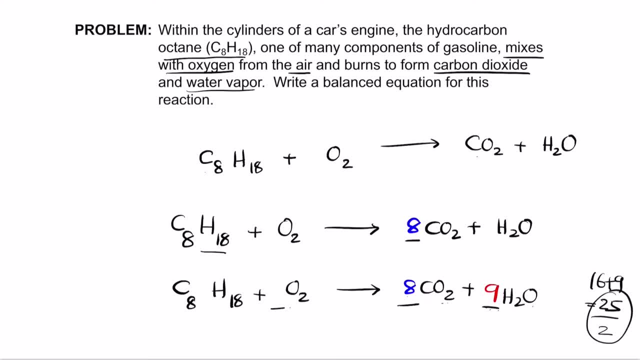 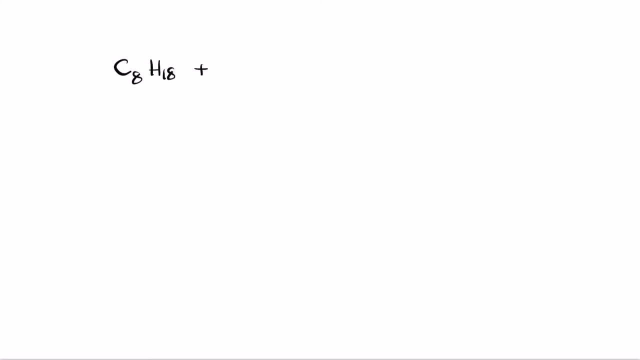 Just divide this by 2.. So whatever the number is, That is the number of oxygen that should be there. So now write down the equation. So C8H18 plus 25 by 2 oxygen gives 8 CO2 plus 9 H2O. 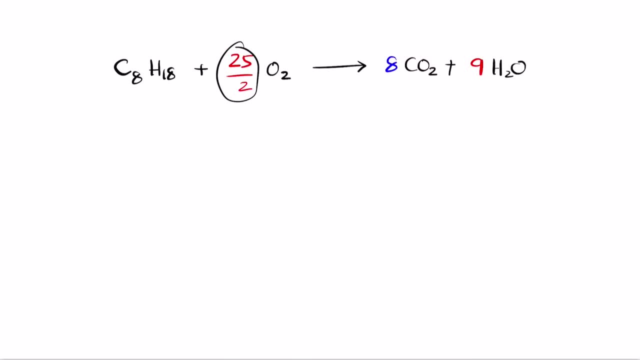 So now we have balance, but this is a fraction, So we do not need, We should not have fractions. So multiply a number so that it does not become, It becomes an integer. So what is the number we multiply here? So multiply the denominator value, which is 2.. 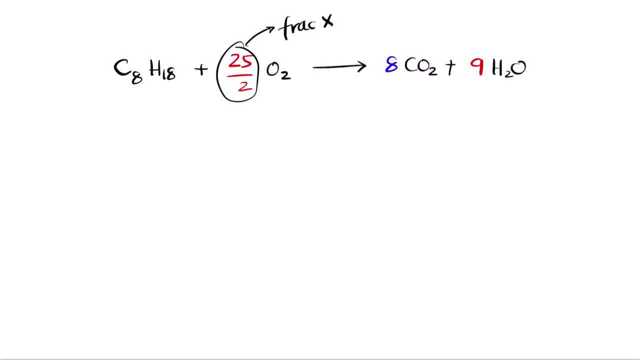 So which gives you the value? So completely, write down the entire value, So that becomes 2 C2- sorry, C8H18- plus 25 O2.. Becomes 8 CO2 plus 9 H2O. So this is the entire part. 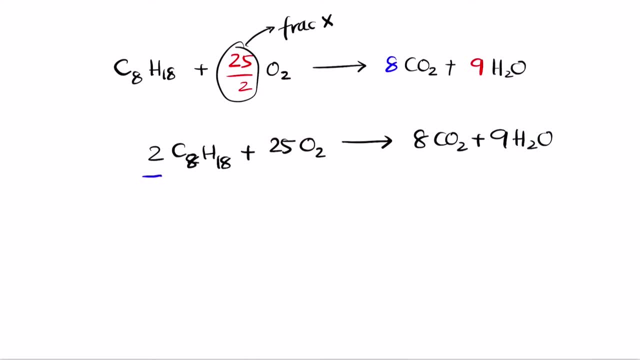 That is completely balanced. So these are the coefficients that we have added into the equation. Now check the number of carbons. There is 16 carbons on this side. There are 30, 6 hydrogens and 50 oxygen here. 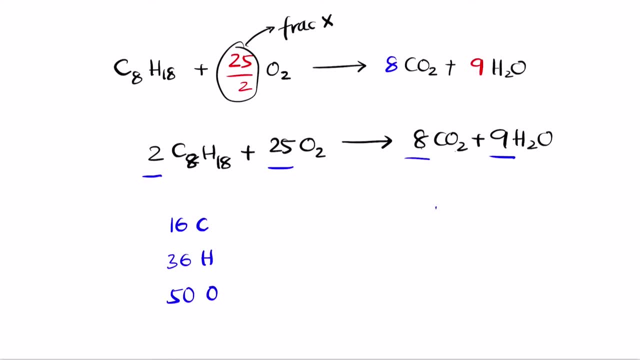 Eight times two, so eight carbons, So 8 to 8.. So when you multiply 2 here, So these two become sorry for that, So these to become 16 carbon dioxide and 18 hydrogen. So when you multiply the entire equation- 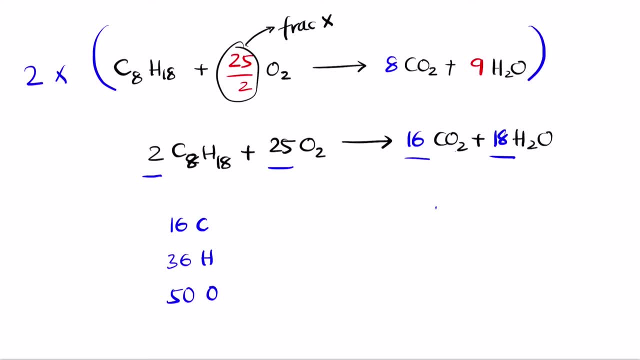 So now on the other side we have 16 carbon, 16 times 16. 16.. to is 36 oxygen plus 18 oxygen, that is 50 oxygen, and you have 36 hydrogen. so 18 times to 36 hydrogen. so both sides there is same number of each of these quantities. so this is balanced. 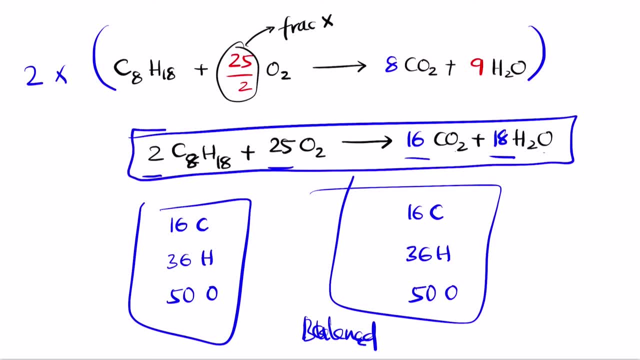 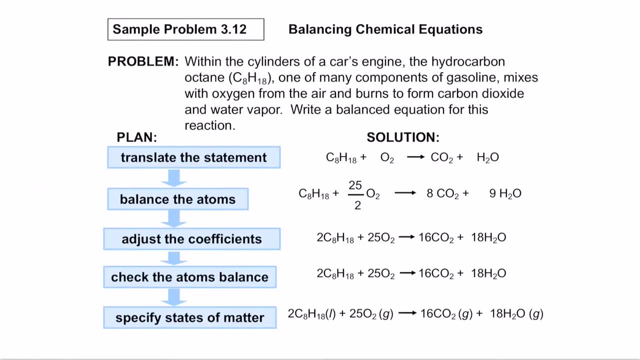 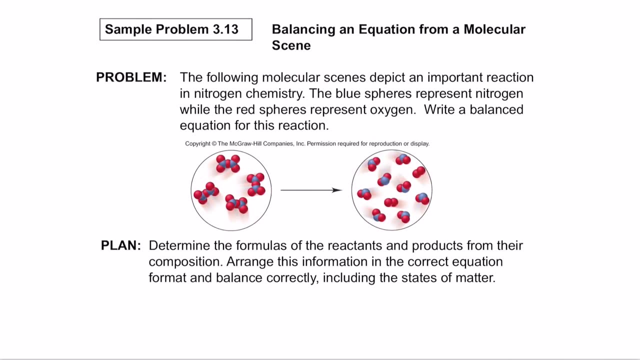 so, and all of them have the least multiples possible. so all of them have the least multiples. so this is the balanced equation. so this is how you balance a chemical equation, right? so this is the molecular scene of the combustion and how the molecules will change now in this. so the following molecules molecular scene depicts an important reaction in nitrogen. 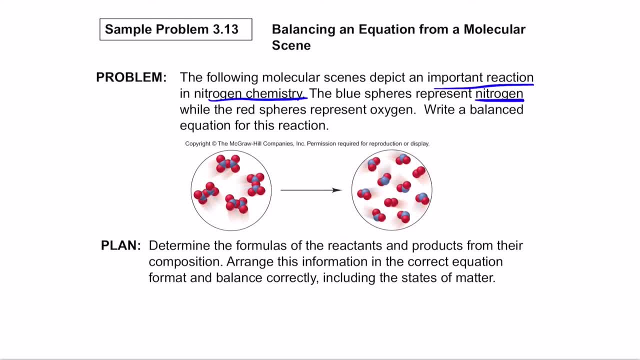 chemistry. so the blue spheres represent nitrogen and the red spheres represent oxygen. so write a balanced equation. so the blue sphere: we want to write the actual molecule that is there. so the blue sphere is nitrogen. there is two nitrogens, so n2, and there is five oxygen o5 gives you have one blue. that is one nitrogen and two oxygen o2. 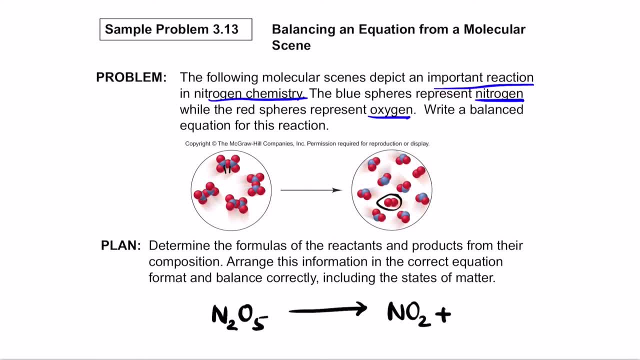 and plus. notice that there are two reds as well, which means there is an oxygen as well. now, on this side we have four of these molecules, so four n2o5, and on this side you have two n2o5. have 1, 2, 3, 4, 5, 6, 7, 8, 8, NO2 and 2 oxygens, so 2. now notice that there is a higher multiple. what is? 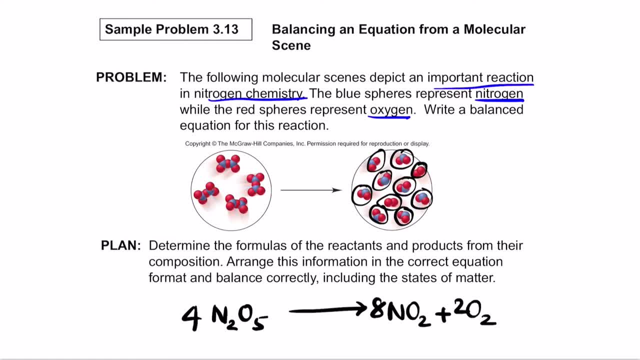 the least common digit divisor that we can use here is find the value that you can divide all of them with, so that is 2. so divide entire thing by 2, so you end up getting the equation: 2 N2O5 gives out 4 NO2 plus O2. so this is the balanced equation for this reaction, remember. 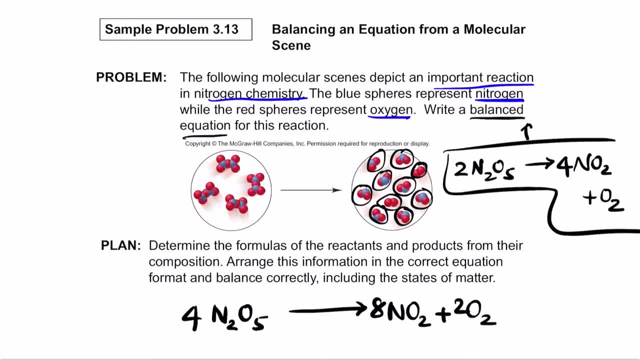 that we need the least common multiple possible. so you do not want to have the entire numbers, so you have to have the least least number of each of these quantities. so the least number possible is 2 N2O5 and 4 NO2 and plus O2. so that is how you get the balanced equation. 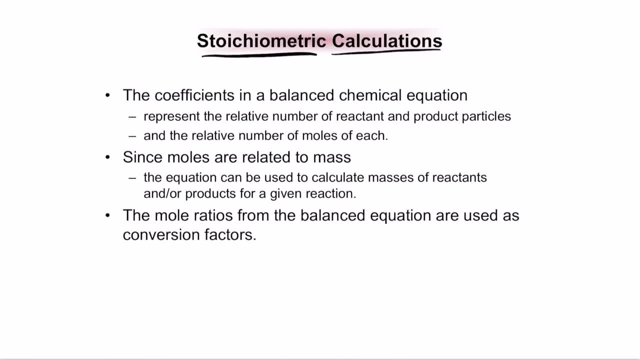 next let us come to stoichiometric calculations. so the coefficients in a balanced chemical reaction also represent the relative number of the reactant and the product particles, and also they represent the relative number of moles of each of these quantities. so since the moles are 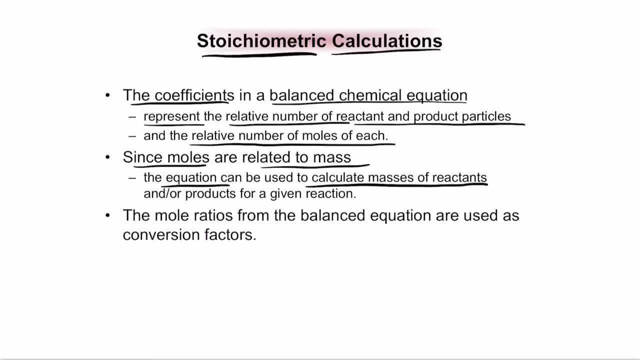 related to mass. so the equation itself can be used to calculate the mass of the reactants and or the products of a for a given equation, given reaction. so the mole ratio from a balanced equation are generally used as connotations, conversion factors. so this is an important point. so the mole ratio is the one that we 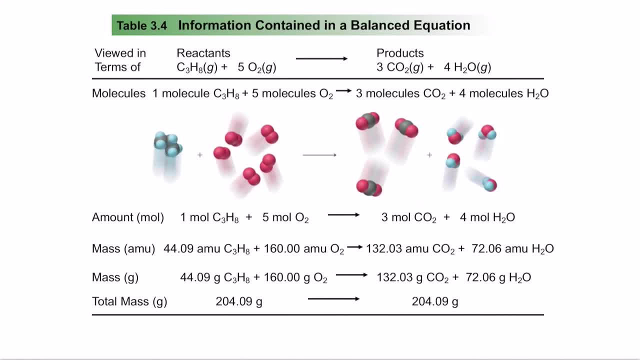 end up using a lot. so let us take a simple example of this to look at a balanced equation. so let us say we have propane mixing with oxygen to get carbon dioxide and water. so 1 mole of propane mixing with 5 moles of oxygen gives 3 moles of carbon dioxide and 4 moles. 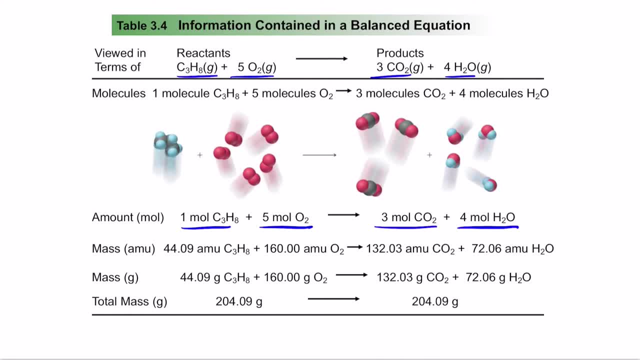 of H2O. which means that when you want to look at this equation, so for 1 mole of carbon dioxide or propane, here you get 3 moles of carbon dioxide, and for 5 moles of oxygen you get 4 moles of water. so this ratios is what we have to remember here. so for 1-5 ratio, you get: 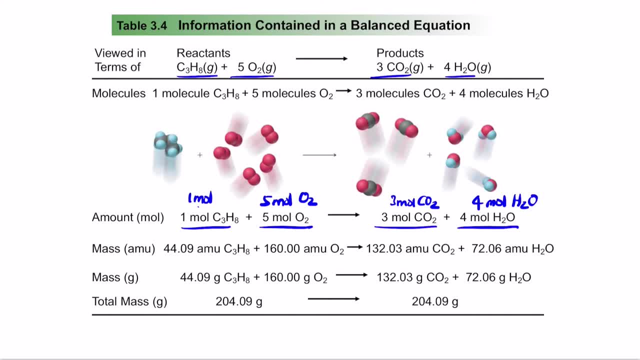 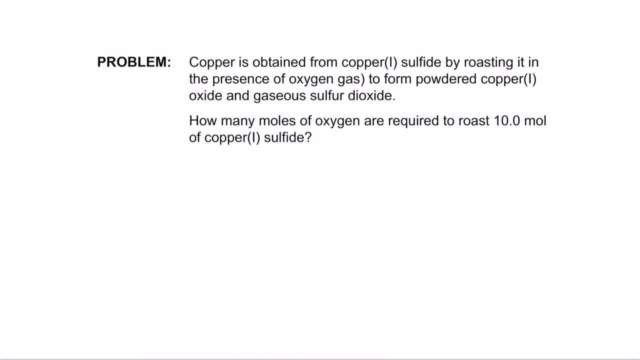 3-4, carbon dioxide, H2O ratio. the same applies to the masses, and the total mass should always be equal to the products. is must be equal to the reactants. so that is the law of conservation of mass. now how do you summarize this equation? so let us take a simple example. so copper. 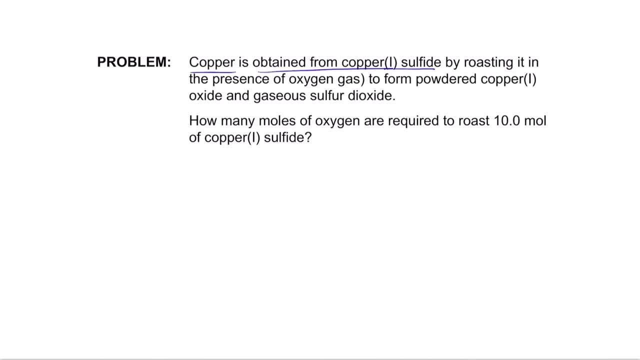 is obtained from copper sulfide by roasting it in presence of oxygen gas to form powdered copper oxide and gaseous sulfur dioxide. how many moles of oxygen are required to roast 10 moles of copper sulfide? so let us try and translate this equation into. let us try to. 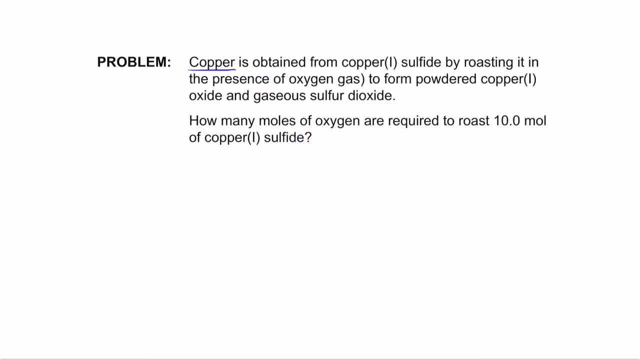 translate this into an equation first. So copper is obtained from copper sulfide by roasting it in presence of oxygen gas. so copper sulfide, so Cu copper sulfide. remember that Cu copper represents Cu plus and S2- sulfur is always 2-, so which means copper sulfide is Cu2S, so they are burning it in presence. 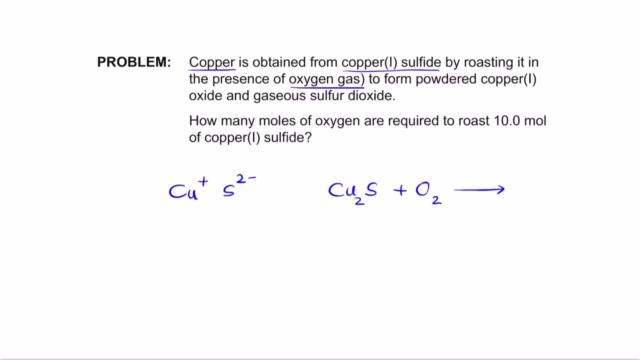 of oxygen. so O2 gives copper oxide, so it burns and provides copper oxide and gaseous sulfur dioxide. Copper one oxide is Cu2O plus sulfur dioxide is SO2. so remember, this is the equation of the general equation that we have. so the first thing we want to do is balance the equation. 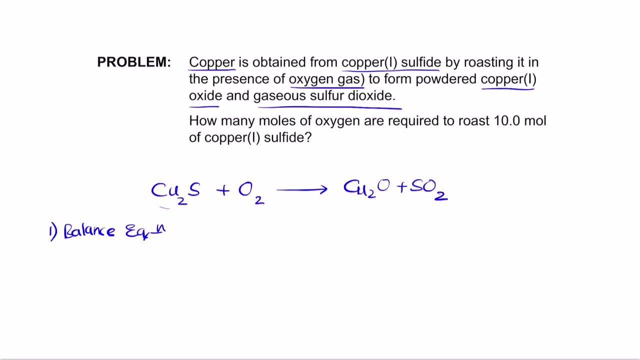 so there are two coppers, two coppers, fine, but there is only two: hydrogen, two oxygens, but there are three oxygens On the other side. so now how to balance this? so balance it based on the number of oxygens. on this side, you have two oxygens. on this side, you have three oxygens, so two are there. 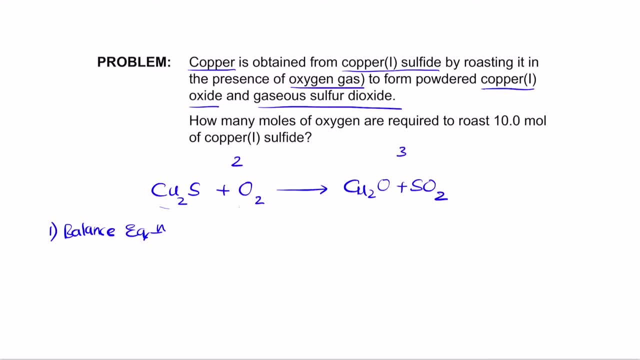 on this side you have three. so cross multiply each of these values with each other, so which means that now you get six oxygens. so how do you get six oxygens now? so write down three oxygens here. So here, When you want to write down, you want to write how many oxygens here. so let's consider that. 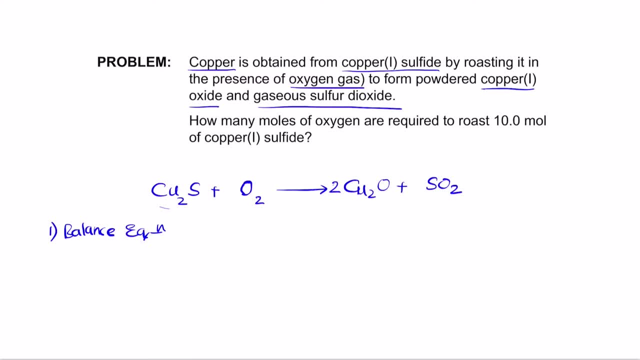 there are two copper dioxide, copper oxides, and there is 2SO2. now that gives you two oxygens plus four oxygens, so that is 3O2. that ends up giving you a total of six oxygens. next you have two sulfur on this side and four copper, so write down two here so that balances. 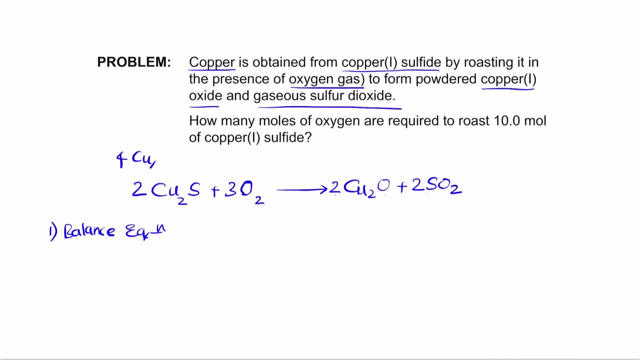 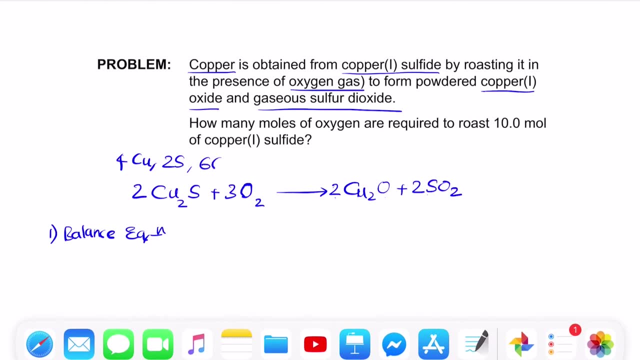 so you have total of four copper. So on the left side you have four coppers, two sulfur and six oxygen. The same thing, you have 4 copper, six oxygen and 2 sulfide. so it's balanced. So now we have balanced the equation. 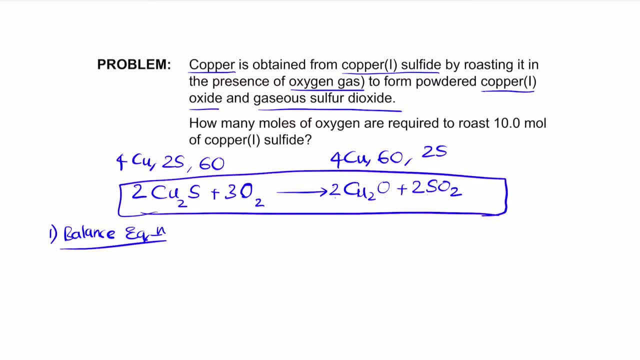 So this is the balanced equation. Now what they are asking you here is how many moles of oxygen are required to roast 10 moles of copper sulfide. So take the ratio. here you have the equation: 2 Cu2s plus 3 O2 gives 2 Cu2O plus 2 SO2.. 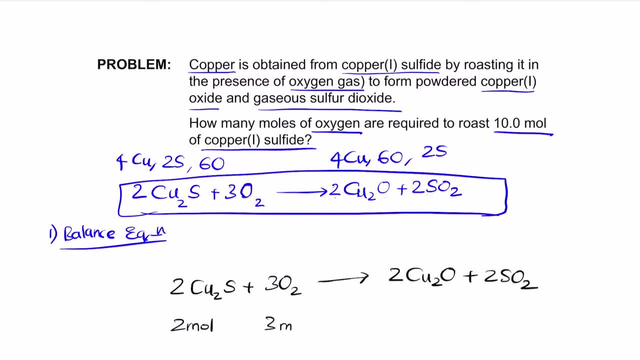 So for 2 moles of copper sulfide you need 3 moles of oxygen to get 2 moles of copper oxide and 2 moles of sulfur dioxide. So write down the ratios that they are asking you for. they are asking you for how many. 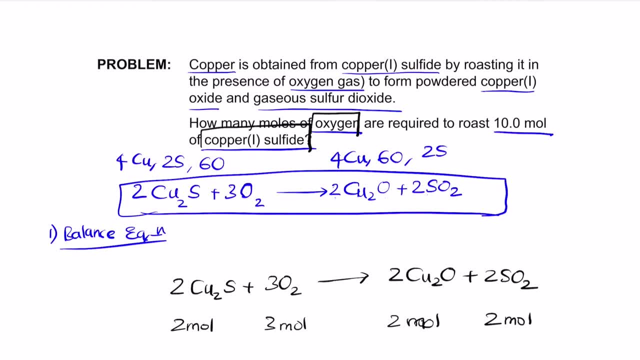 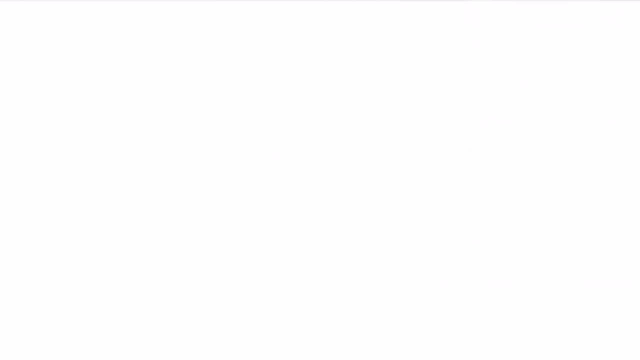 moles of oxygen is required for 10 moles of copper sulfide. So write down just copper sulfide and oxygen ratio. So from this we can write. for 2 moles of Cu2s You need 3 moles of oxygen. 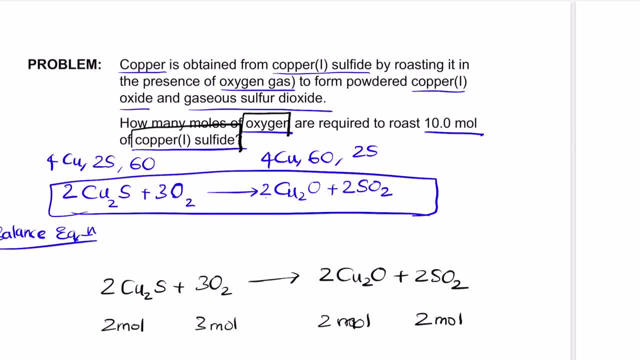 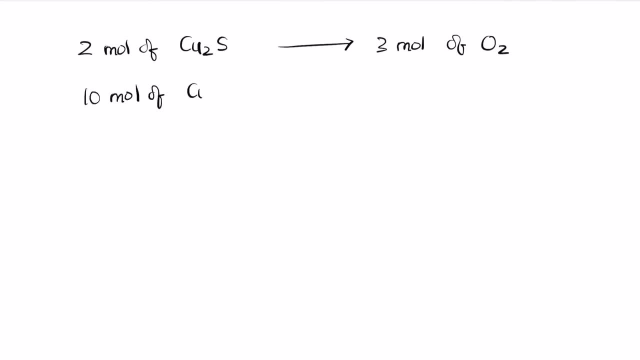 In the question they are asking you: they have 10 moles of copper sulfide, and how many moles of oxygen do you require? So 10 moles of copper sulfide, and they are asking you how many moles of oxygen is required. 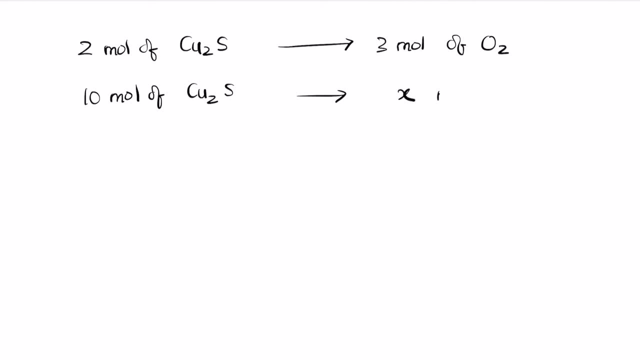 Let us consider that this ratio here is some value: x, so x mole of oxygen. How do you find the answer? So cross, multiply and equate the values. So multiply here, cross, multiply. So 2 times x becomes 3 times 10.. 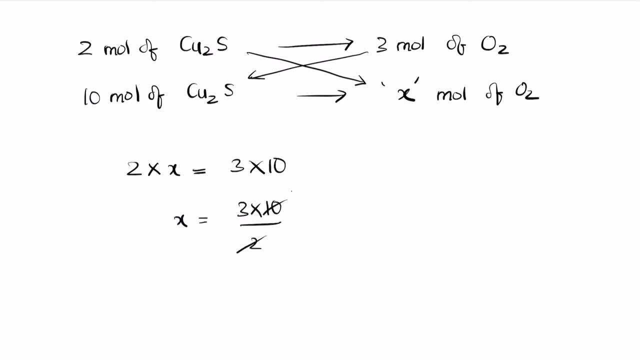 So x becomes 3 times 10 by 2.. So 2 times 2 1's, 2 5's, so you get 15 moles. So which means that for 10 moles of Cu2s you need 15 moles of oxygen. 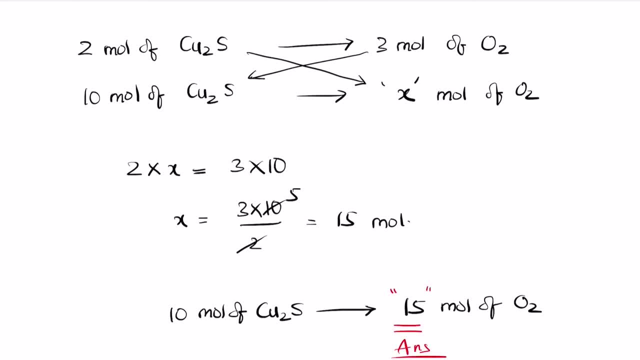 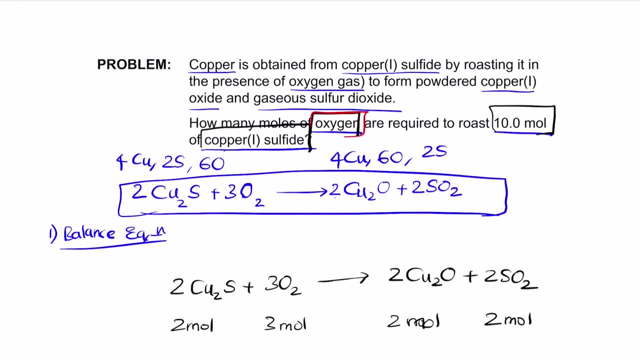 So this is your answer. So I hope you understand how to find this. Remember what are the values that they are asking you here. They are asking you for the ratio between oxygen and copper sulfide. Use the ratio from the equation and try to translate that into the equation that they 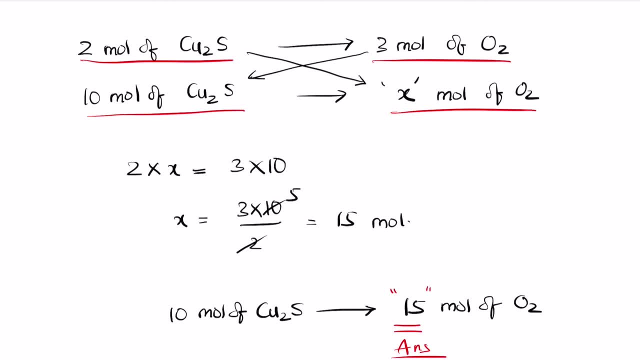 are asking you for, And cross, multiply and equate the values. That is when you get your final answer for whatever the value that you have. So this is how you can solve using stoichiometric calculations. So let us try the same problem, but let us use different parts. 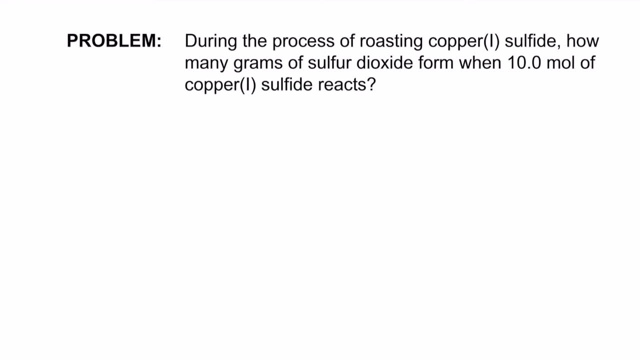 So again it is the same thing: roasting of copper sulfide. So you have Cu2s. So 2 Cu2s plus 3 O2 gives 2 Cu2o plus 2 SO2.. Now here they are, asking you for how many grams of sulfur dioxide will form for 10 mole. 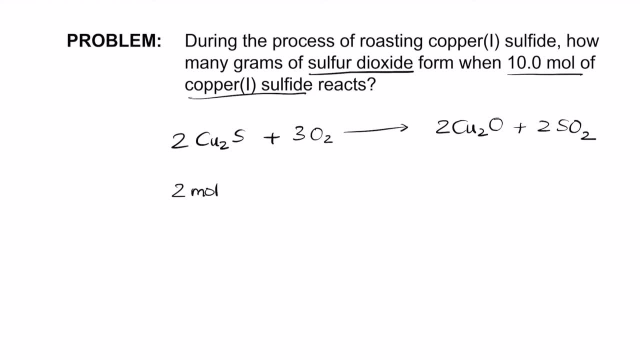 of copper sulfide. So here, 2 moles of copper sulfide, you get 2 moles of sulfur dioxide. So, but they are asking you when you have 10 moles of copper sulfide. So lets consider that there is X moles of SO2.. 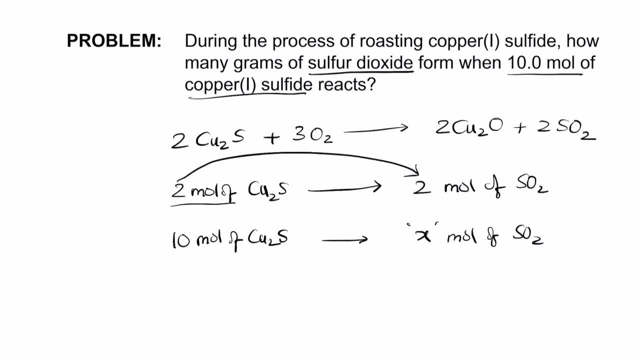 If you notice that the ratio is the same, 2 will give 2, which means 10 will also give 10.. You can also try the other method of cross multiplying. So 2 times X is 10 times 2.. X becomes 20 by 2.. 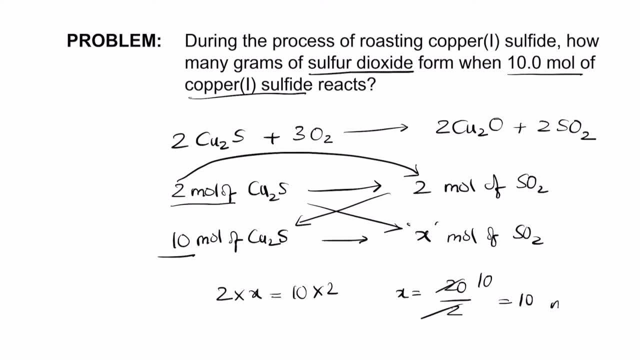 That is the second together. 2- you still get the same answer. so for 10 mole of copper, 1 sulfide, you get 10 mole of sulfur dioxin. so this is your answer. so remember that the balanced equation is what you need to solve these problems. 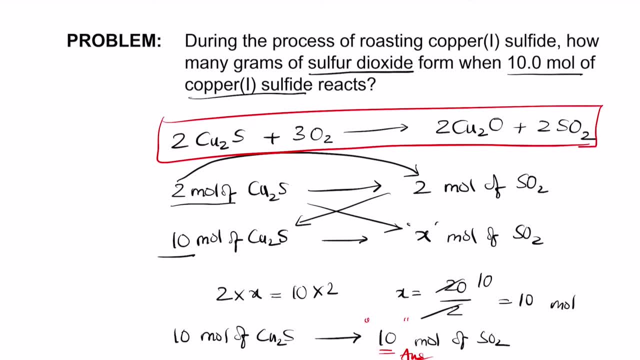 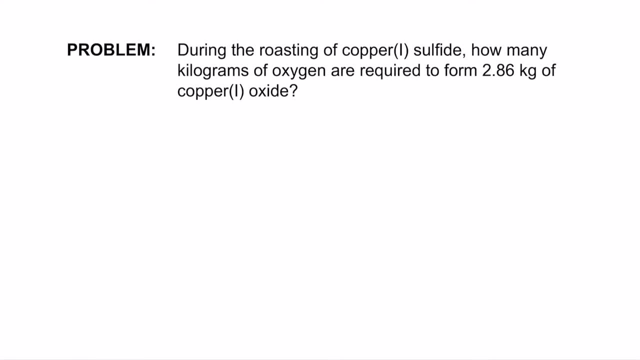 so if you don't balance it correctly, then you will not get the right answer. so what to do if, rather than giving you the values of mole, they have given you the mass? so again, use the same thing, but first things first, try to note down the balanced equation. 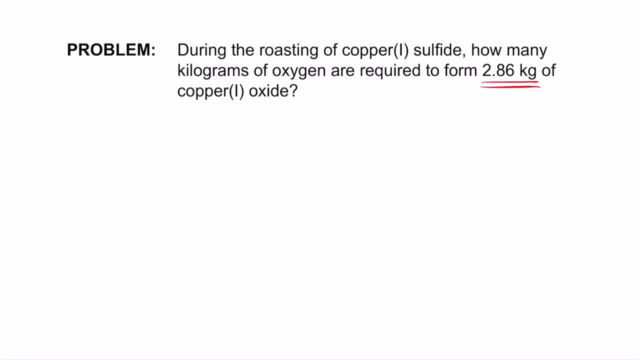 so the balanced equation is: 2 CO2S plus 3 O2 gives 2 CO2O plus 2 SO2. now, this is the equation. now, using this equation, first thing they're asking you is: they have 2.86 kg of copper oxide, so this: 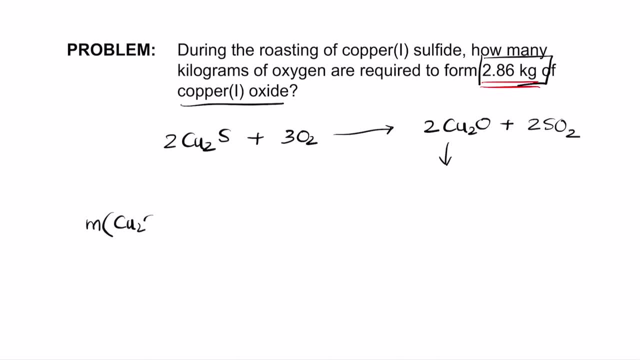 is the mass they have given. so they've given the mass of copper oxide, which is 2.86 kilograms. so whenever they give you mass, convert it into grams. so 2.86 kilograms into 1000, so 1 kilogram is 1000. 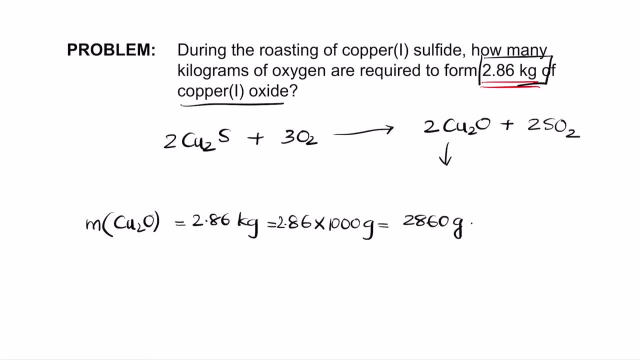 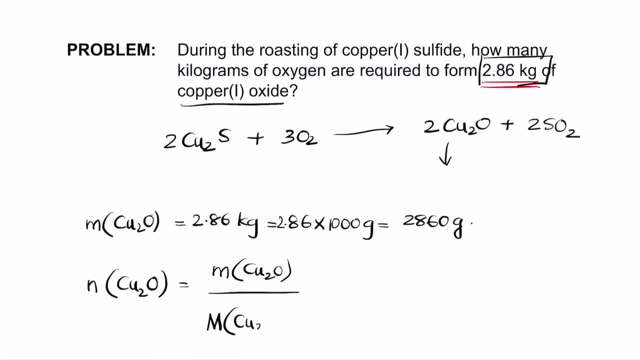 divided by the molar or mass of copper oxide, so the mass of CO2O is 2 860 by now. we want to know the molar mass of copper oxide, so the molar mass of copper is 63 point 5, 5. oxygen is 16.06. so you want to find the molar mass of CO2O, so that is gonna be 63 point 5 pcs. 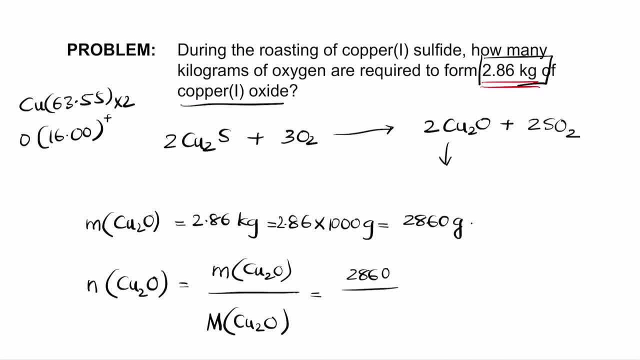 plus 60. So you have 63.55 times 2 plus 60. So that value is 143.1.. So that is the molar mass of copper oxide. So you can try using the you know calculator and try to calculate it. 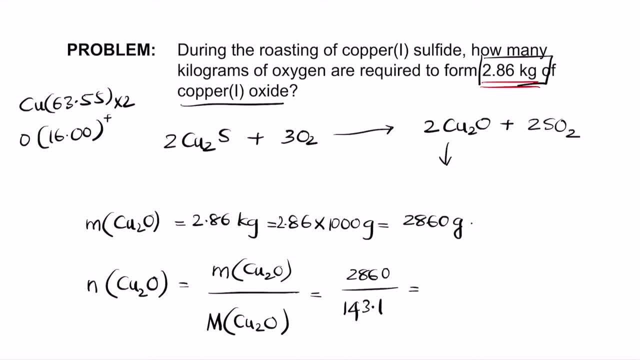 So now try to calculate the number of moles. So 2860 over 143.1.. So that gives you a value of 19.986 mole of copper oxide. So this is the moles here. Now the relationship they are asking. 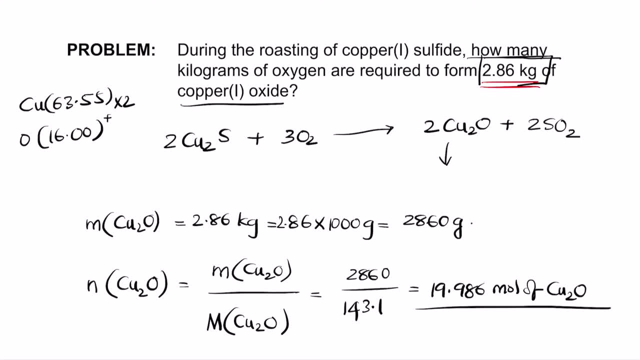 is how many kilograms of oxygen are required to form 2.86 kilograms of 2 kilograms of copper 1 oxide. So they are asking you the relationship between oxygen and copper oxide. So they are asking for relationship between oxygen and copper oxide. So for every 3 moles, 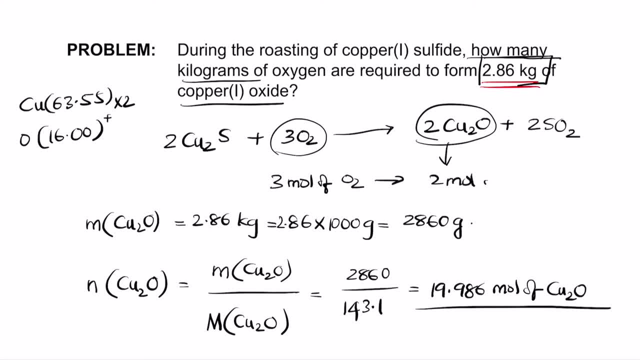 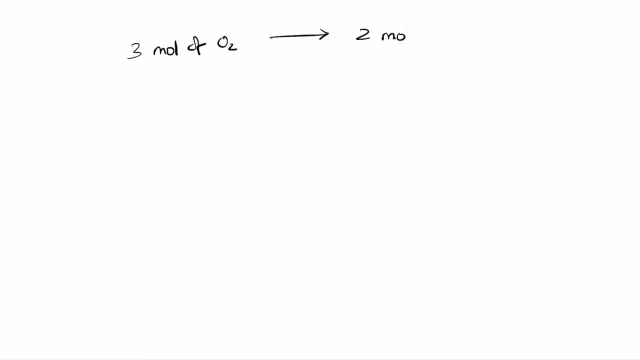 of oxygen, you get 2 moles of copper oxide. Now let us use the ratio itself to get the answer. So for every 3 moles of oxygen, you get 2 moles of copper oxide. Now the total number of moles. 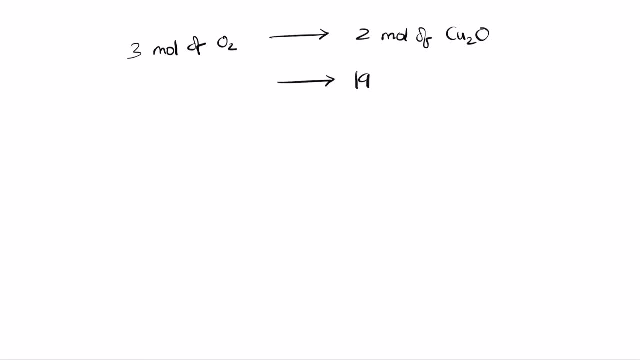 of copper oxide. now write it down as the ratio here. So that is 19.9.. Let us get that 22.996 mole of copper oxide For that. what is the x mole of oxygen? Let us find the number of moles first. So what is the moles of oxygen now? So cross, multiply again. So 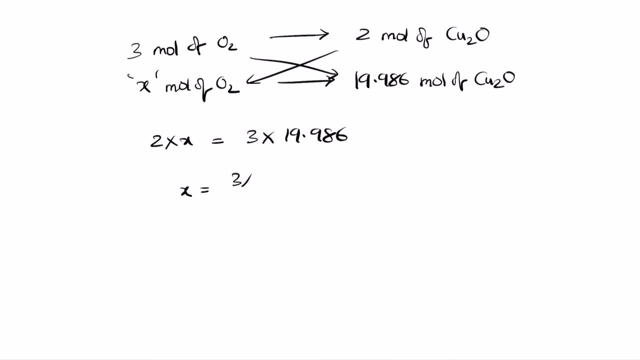 2 times x becomes 3 times 19.986.. So x becomes 3 times 19.986 by 2.. So the value is 29.996,. ok, So, guys, then what will you do? You have to do 32,000 times the resistance, tremendous tool. 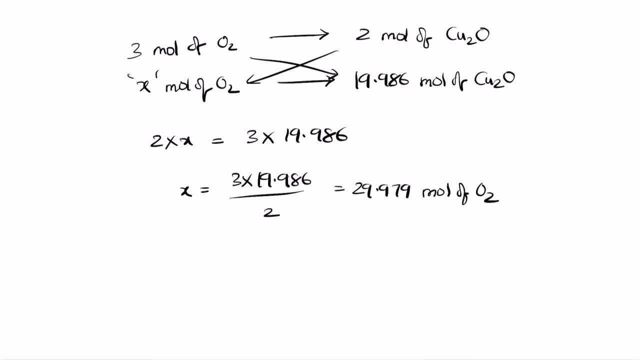 nine, seven, nine mole of oxygen. but the answer that they are asking you is not in mole, they are asking you in kilograms. so they are asking you for the mass. so we know that the number of moles is mass by molar mass. if you want to find mass now it becomes number, the number of moles. 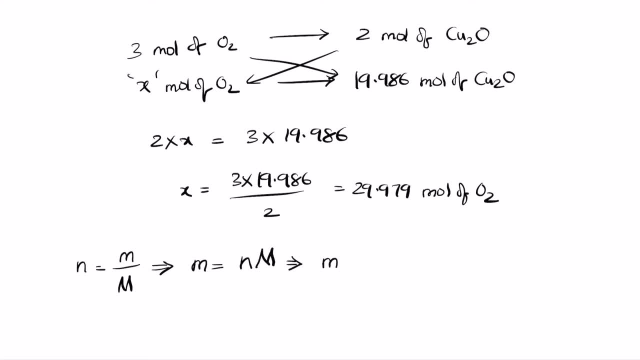 into the molar mass. so we want to find the number of mass of oxygen. so it becomes the number of moles of oxygen times the molar mass of oxygen. the number of moles of oxygen is 29 point. so this is the value here: 29.979 times the molar mass of oxygen will be 32.00. notice that each oxygen is 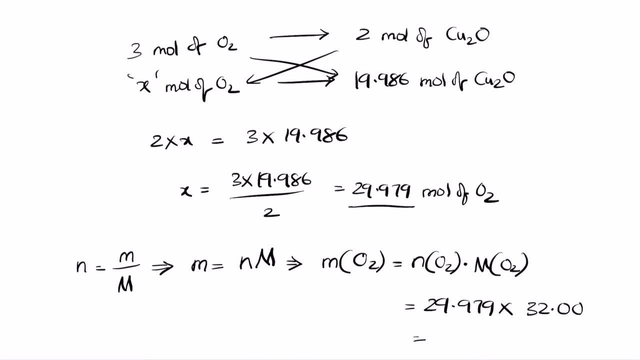 16, so two of them are there- 32. so multiply 32, you get 959.329 grams. so this is the mass of oxygen that you need: 959.329 grams. remember that everything that you get using the atomic table is a periodic table, is. 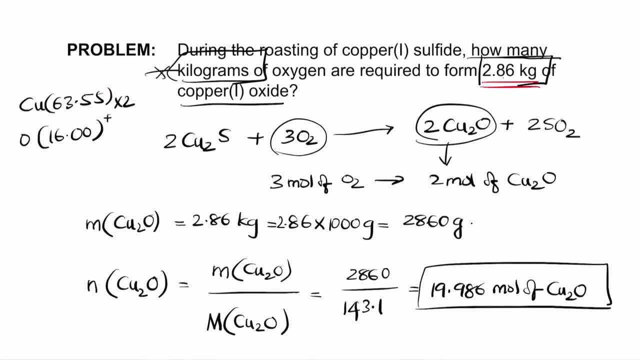 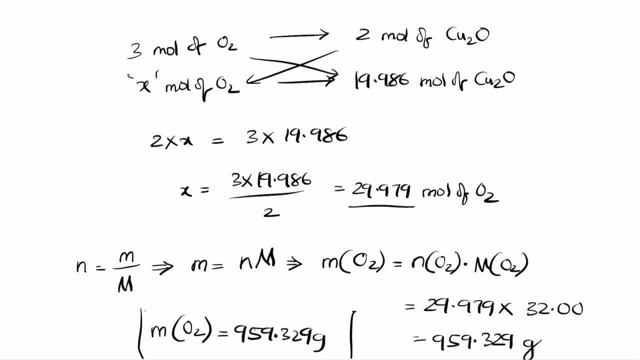 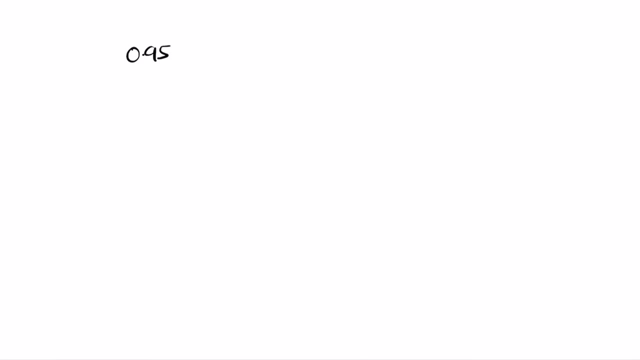 always in grams. now they will ask: not ask you in grams, but they've asked you in kilograms. now how to find it in kilograms now? so this is going to be: divide this by 1000, that's you get 0.959 kilogram. so when you use 0.959 kilogram of oxygen, you get 2.86 kilogram of copper oxide. 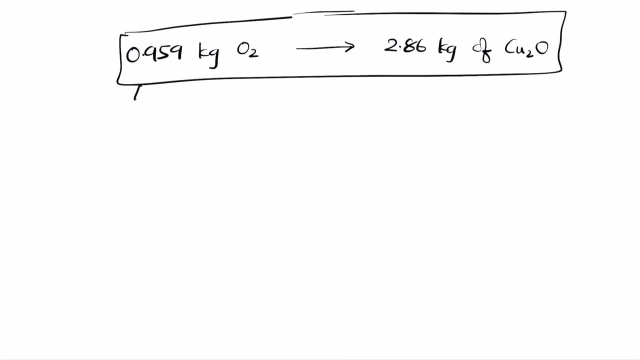 so this is your answer. so this is how you can use: from mass you can go into the number of moles. from moles again you can come back to the mass. so let's try another example of this and let's see if you can solve this. 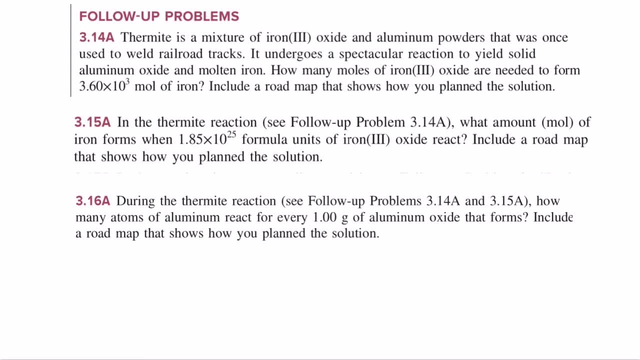 so try this problem on your own and see if you can get notice that here. termite is a mixture of iron three oxide and aluminum powder that was once used to weld railroad tracks, so it undergoes a spectacular reaction to you: sodium, aluminum oxide and molten iron. so how many moles of iron three? 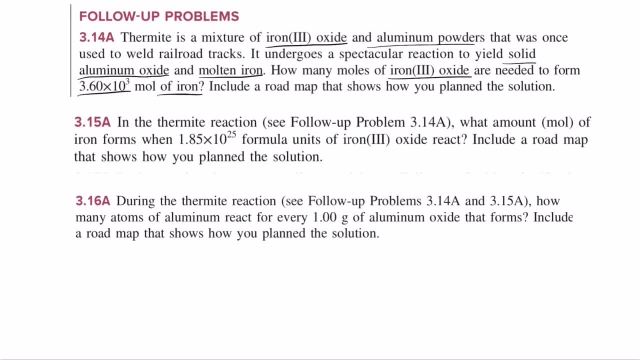 oxide are needed to form dash moles of, so this moles of iron. so here they are, looking at a reaction of iron three oxide. remember iron three is Fe3, oxygen is O2 minus and aluminum is Al right. so we are looking at Fe2O3 plus Al forms, aluminum oxide and molten iron. so Al2O3 plus iron, molten. 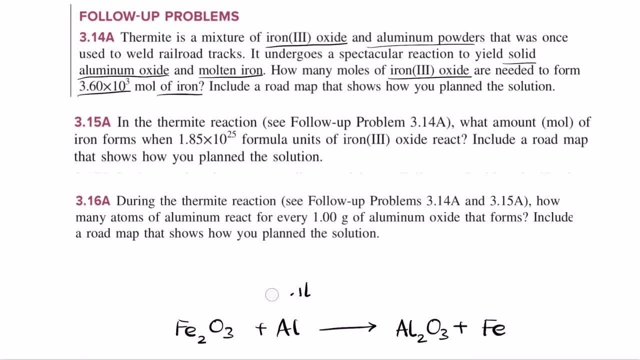 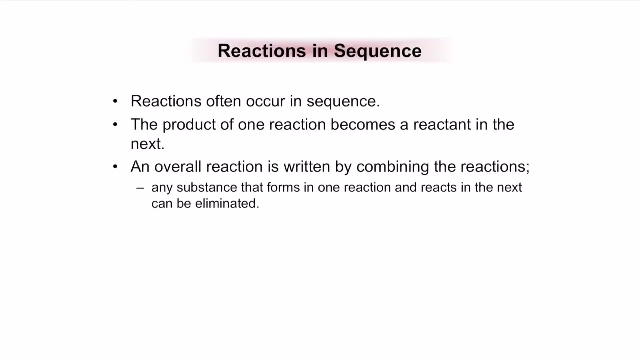 iron is Fe, so how would you balance this reaction now? so try to balance it first. so this is the reaction of this problem. so try balancing the equation first and try to solve the problem using the balanced equation. so pause the video right here and try to solve this problem so generally. 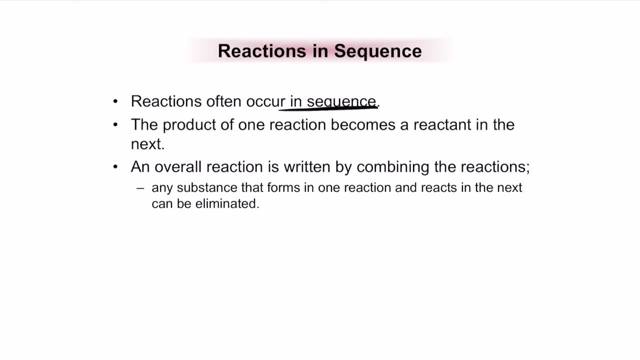 chemical reactions often occur in a sequence, so the product of one of this to one of the reactions becomes the reactant in the next, next reaction. so whenever we write this, we write an overall reaction. so overall reaction is basically written by combining all the reactions that are generally done. so it means that any substance that forms in 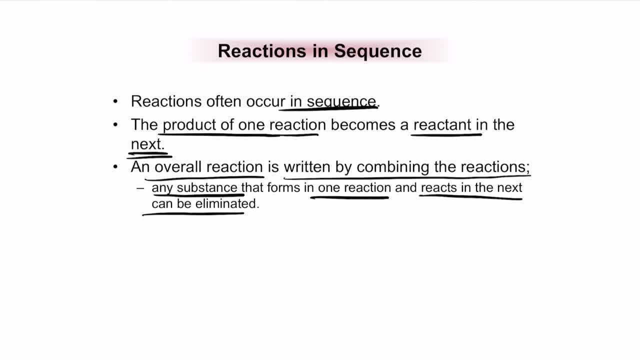 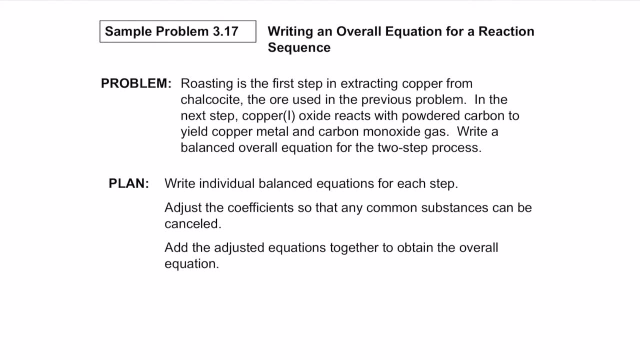 one reaction and does not react in the next, so can be eliminated. so let's take a simple example. let's take the reaction that we already used before, and in that reaction we ended up forming. so copper one sulfide reacts with oxygen to form copper one oxide and sulfur dioxide. so this is. 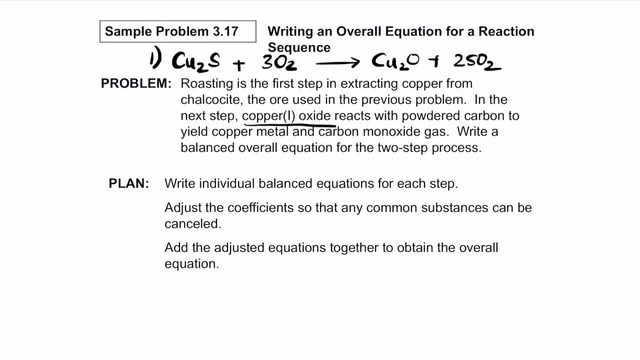 the first step of the reaction. in the second step, copper-oxide reacts with powdered carbon to yield copper metal and carbon monoxide. so then, in this step, copper- one oxide reacts with powdered carbon- is carbon must see gives copper meddle plus carbon monoxideCO. How will you balance? 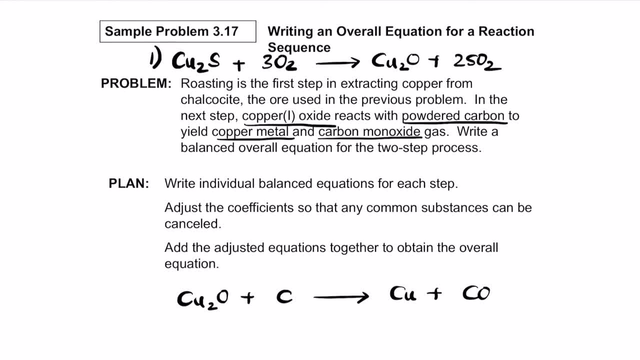 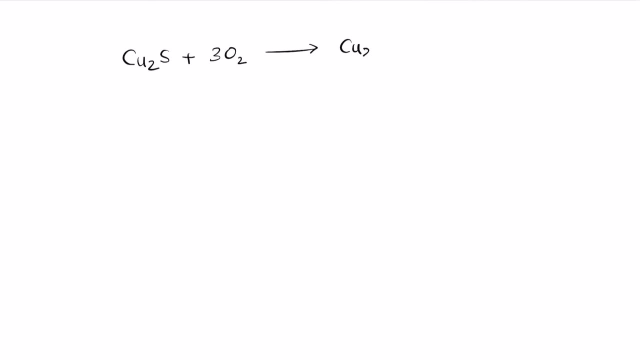 this reaction: there is two copper here and there is only one copper there. so right, two copper. so notice that it's already balanced. not combine both the reactions in the next step. So you have CO2S plus 3O2 gives CO2O plus SO2, so this is the balanced equation. 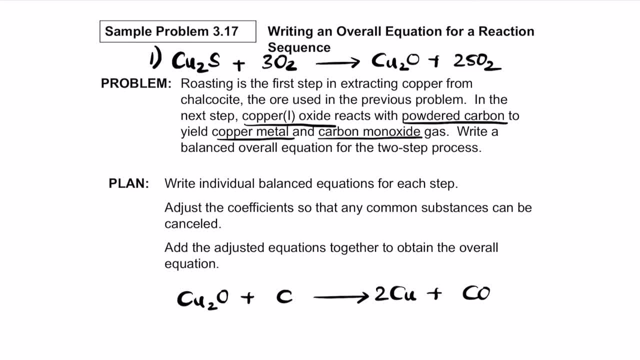 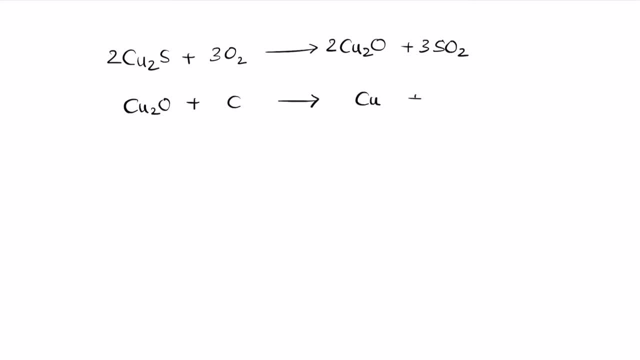 Now in the next step, we have: CO2O plus C gives 2CO plus. so CO2O plus C gives CO plus 2CO. right, so 2CO plus CO. but notice that there are two copper oxide ions here there. 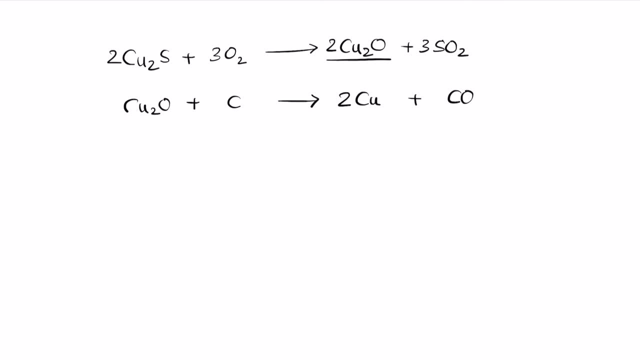 is only one that is being used. So what do you do here is you have to use the entire thing. so when you write the balanced equation, whatever the ones that are common in both of them should have the same coefficient. So here, CO2O is the common one in both of them, so both have to be having the same coefficient. 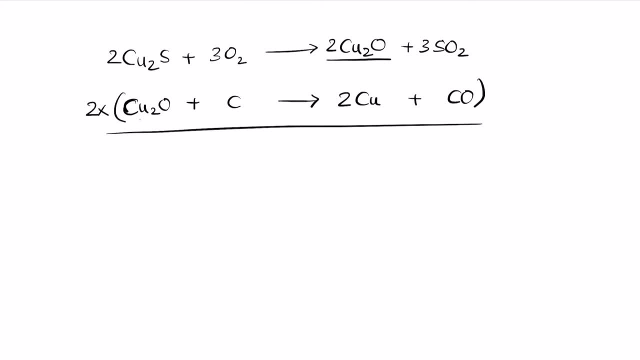 so, which means that multiply this entire equation. So now you get CO2S plus 3O2, gives 2CO2O plus 3SO2, now, whatever is the total amount used in the second equation- 2CO2O plus 2 carbon- it gives 4CO plus 2CO. now cancel. 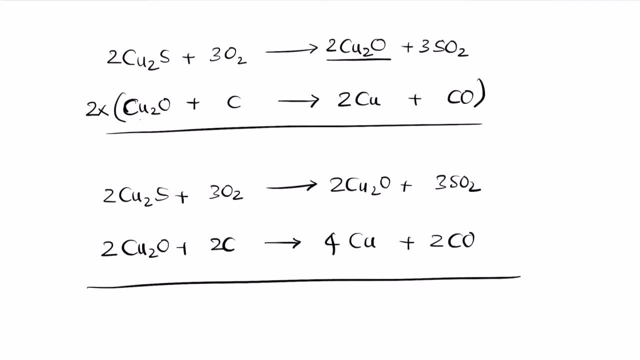 the common ones on each side. so the common ones on each side is 2CO2O and 2CO2O. right Now, write down the balanced equation in full. So write down the everything on the reactant side. write down everything on the product. 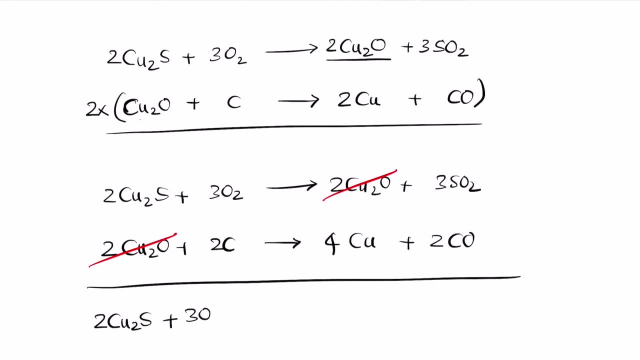 side. So 2CO2S plus 3O2 plus 2 carbon gives 3SO2 plus 4 copper plus 2CO. This here is an example of overall reaction. so where we combine multiple reactions, so we combine two reactions to get one final reaction. 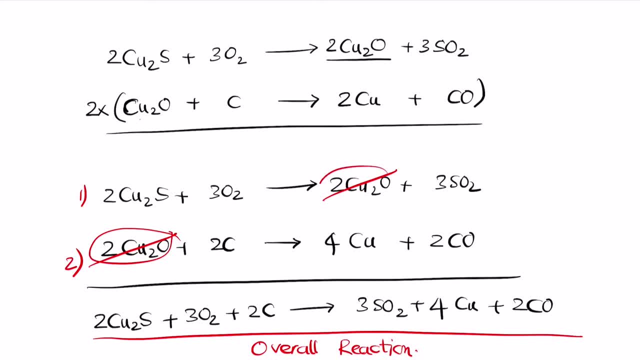 So CO2O. So CO2O here is called an intermediate, so it is also called the reaction intermediate. so it is generally called the reaction intermediate. this is the one that occurs in the middle of the reaction but never forms the final compound, so this is called as an reaction intermediate. 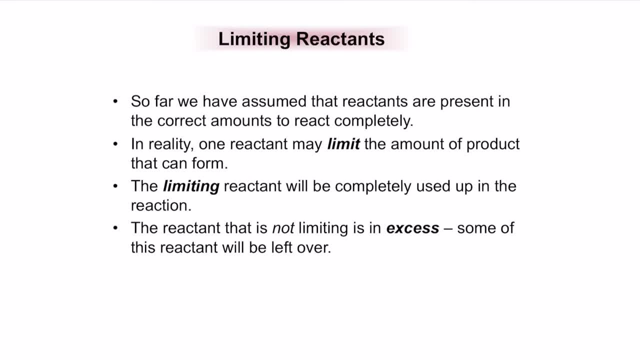 So this is how we write the reactions. The next one is to understand what is the limiting reactions. so what we assumed until now is that the reactants that are present, The reactants that are present, are always in the correct amounts to react completely. 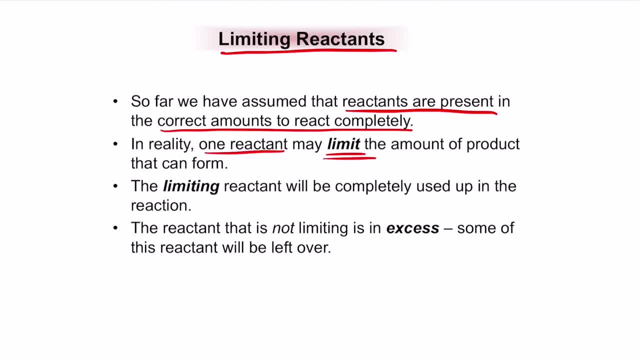 but in reality one reactant will generally can limit the amount of product that can form. so that reactant that can, you know, limit the product formation, is called as the limiting reactant. So the limiting reactant is the one that gets completely used up in the reaction and 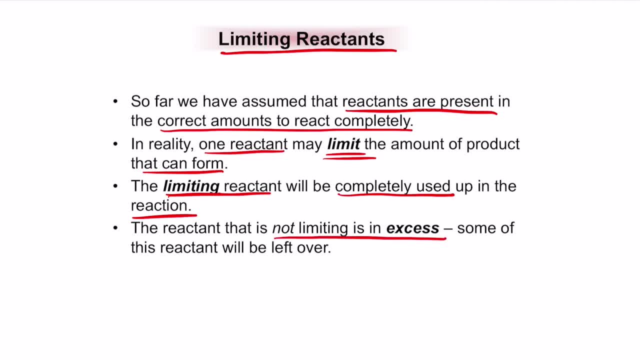 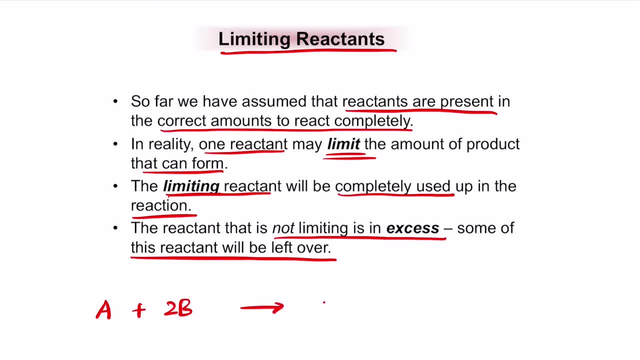 So let us say A plus 2, B forms AB2.. If A is complete, B will not react with anything else, which means that the product also cannot form. so here A is called as the limiting reactant. so by using stoichiometry we can. 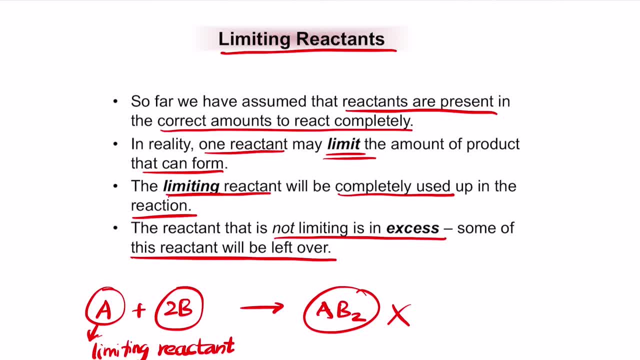 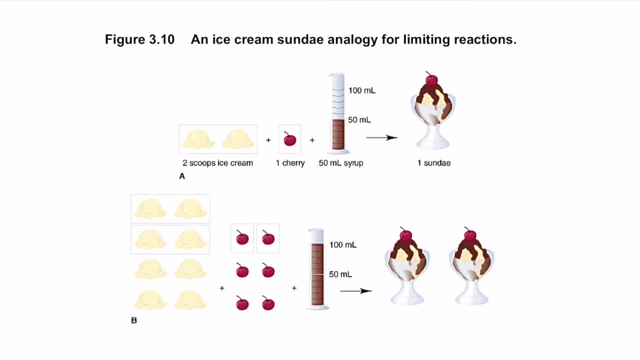 detect whether a given reactant is a limiting reactant or not. So let us take an example of that: EO is a limiting reactant, to look at the analogy of an ice cream sundae. so when you want to create one ice cream sundae, you need two scoops of ice cream, one cherry and 50 ml of syrup. 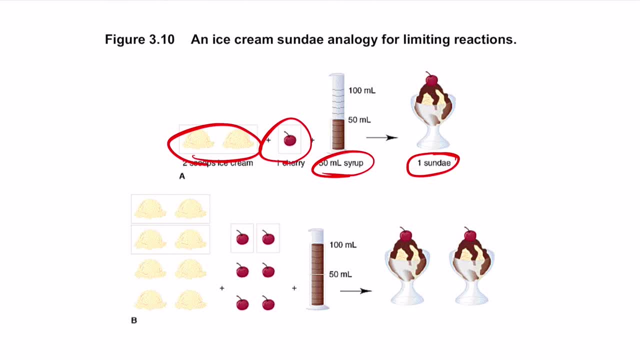 and let's say. the other one is that let's say we have eight scoops of ice cream, six cherries, and you only have a hundred ml. now the maximum number of sundaes that you can make is only two sundaes. the reason is because you will. 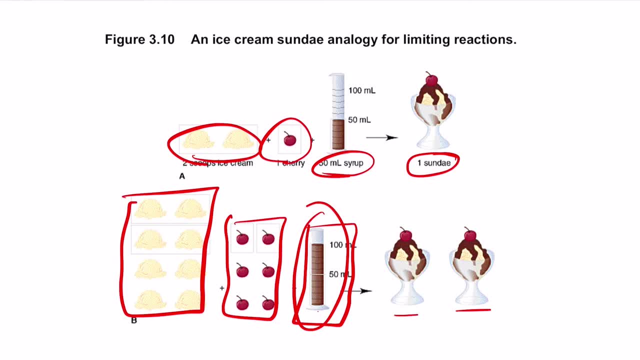 end up using up the entire chocolate syrup here. so which means that this syrup is not if sufficient. even though you have scoops of ice cream and cherries, you cannot create sundae because syrup is missing. so here syrup becomes the limiting reactant in this reaction. so this is how you understand. 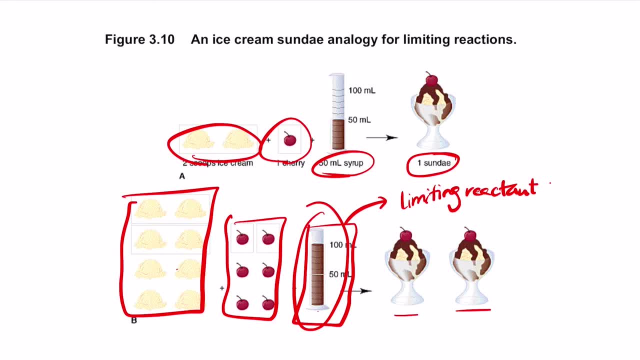 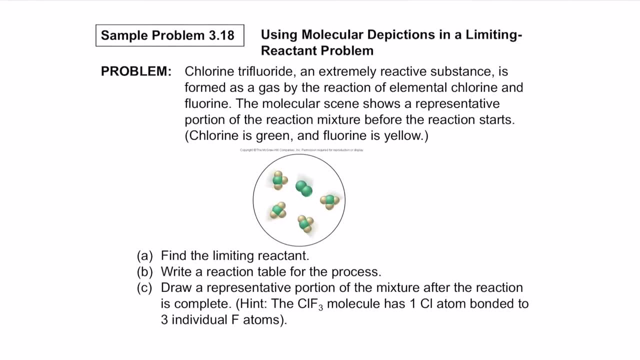 the topic of limiting reactant. so when one of them is complete, the others cannot react and form the product, so that one is called as the limiting reactant. so let's take an example here. so chlorine trifluoride is an extremely dangerous substance and it is a very dangerous substance and it is a very 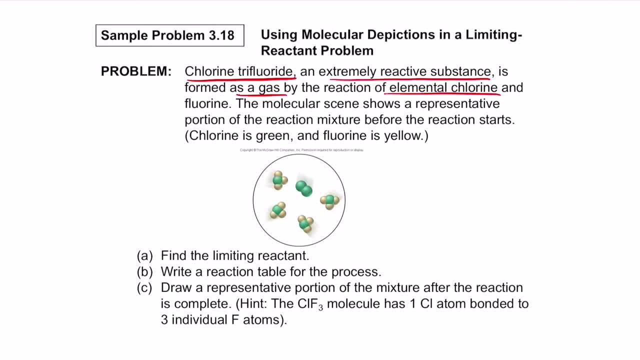 reactive substance formed by a gas, by a reaction of elemental chlorine and fluorine. so the molecule is seen here shows a representation of the portion of the reaction mixture before the reaction starts. so here chlorine is green and fluorine is yellow. so they're asking you to find the limiting reactant. so 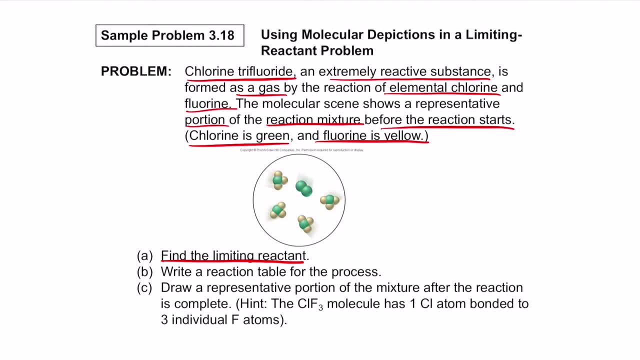 remember, the reaction is between chlorine and fluorine. so you have Cl 2 and F 2. so if you want to write down the reaction, we can write it as so: Cl 2 plus F 2 gives Cl F 3. so if you want to balance the equation, we get you know 3 F. 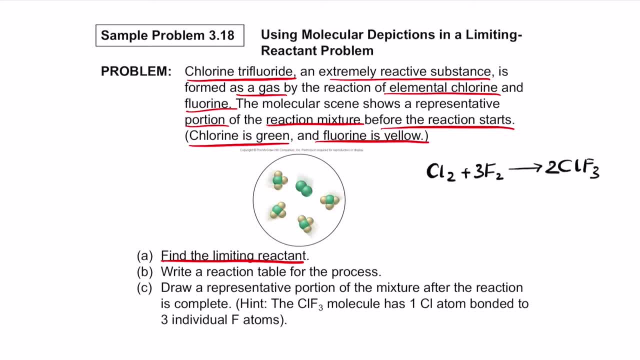 2 and 2 Cl, F, 3, so that balances the equation. but now the question is: if you look at the reaction, which of these is the limiting reactant? so notice the total amount of parts that are used up. so remember that if it is left out, it's. 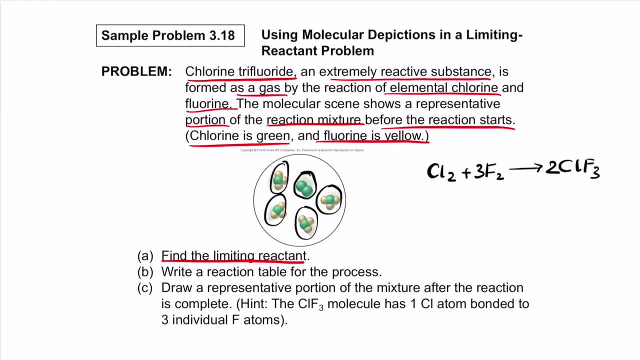 not the limiting reactant, so which is completely utilized here in this reaction? so the one that's completely utilized is fluorine, because there is no fluorine left by itself. remember, fluorine is two yellows, so those two yellows are not present here. fluorine is the limiting. 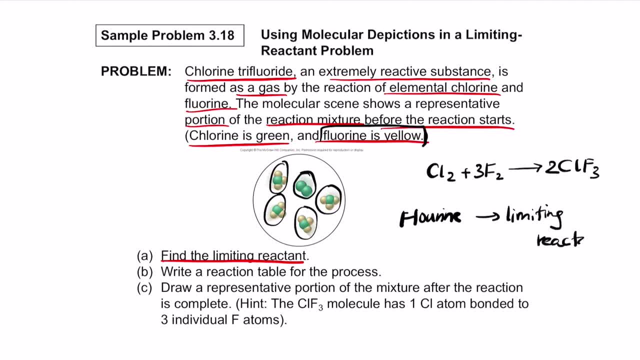 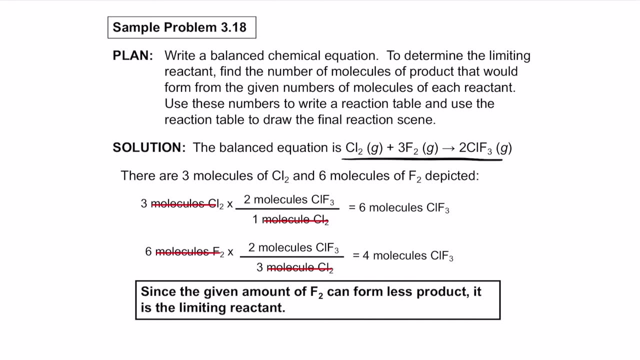 reactant, right? so the one that gets completely utilized is called as the limiting reactant. so write a reaction table for this process. so how will you write the reaction table for this process? so the first thing is to write down the balance equation. so now let's note down the reactant itself. so how would you write this is? 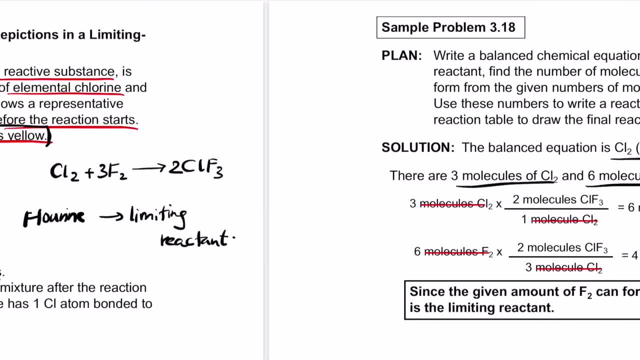 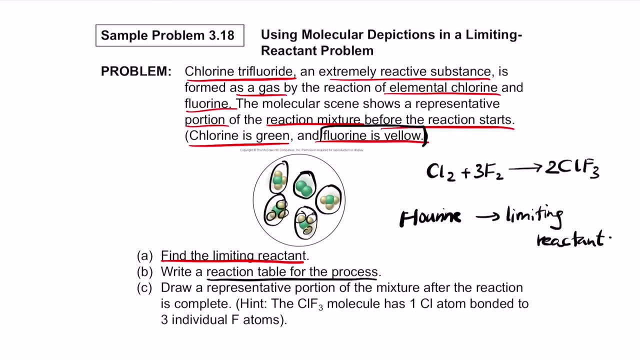 there are three molecules of chlorine and six molecules of chlorine that are depicted in this reaction. so you have a total of one, two, three, four, five, six, seven, eight, nine, ten, eleven, twelve, so that is twelve fluorine and six chlorepo irm, so there are sixoring depicted at twelve. 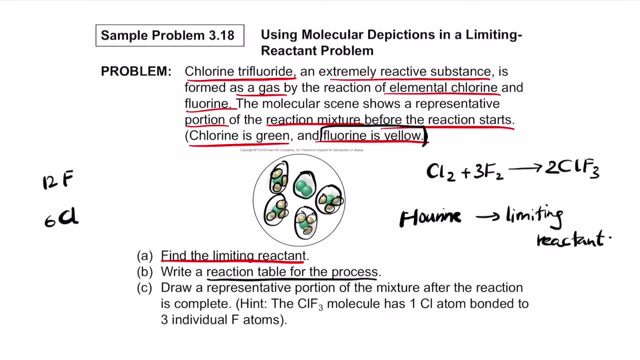 depicted. if you write the actual element, the molecule form. so you write you have three chlorine molecules and six chlorine molecules. so when you write the reaction notice, the reaction here is to note down how many products will you get. so when you want to write down in the 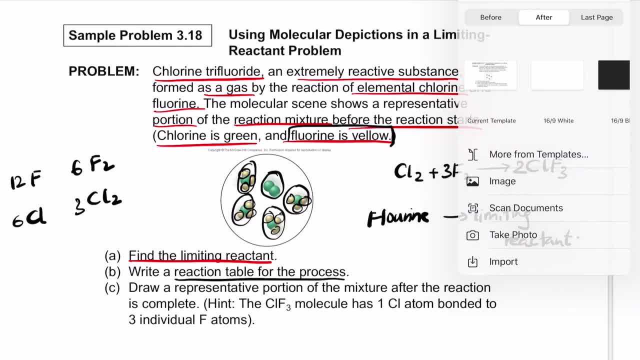 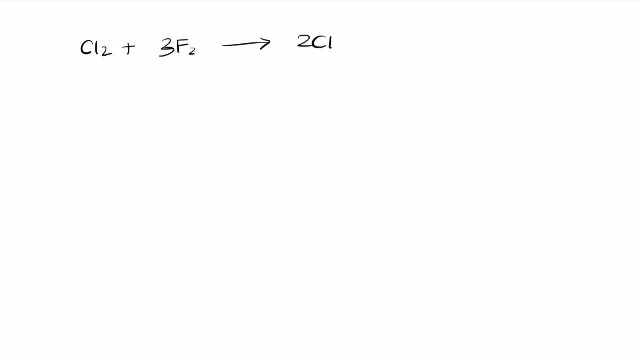 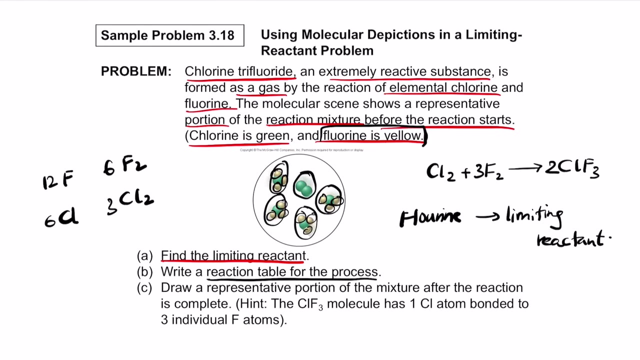 reaction for one mole of chlorine. so we have cl2 plus 3f2 becomes 2cl- f3. so for one mole of chlorine we need three moles of chlorine and two. you get three moles of clf in the reaction. we have six moles of fluorine and three moles of chlorine, so we have 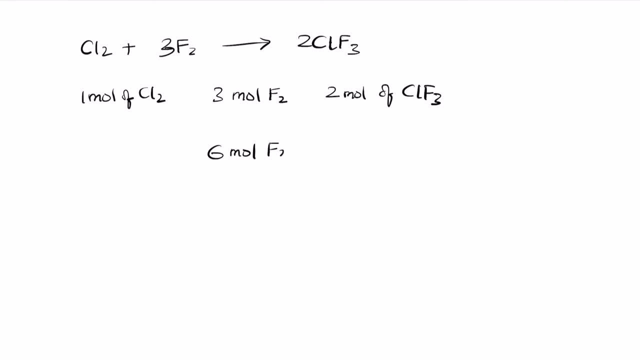 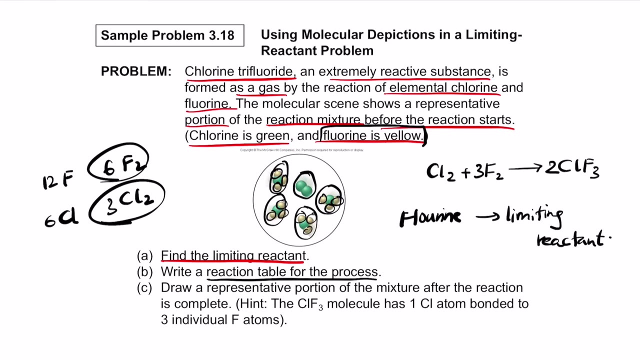 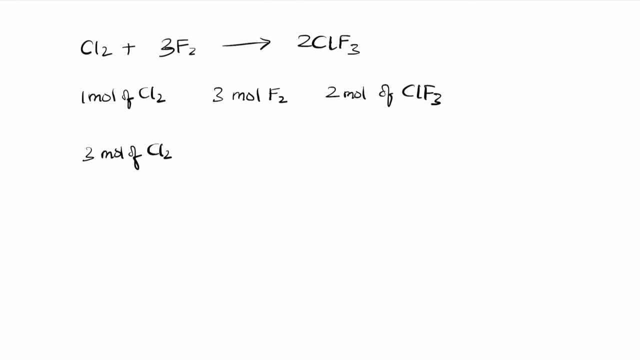 six moles of chlorine and three moles of chlorine. so which means now we have to, we have to know what would be the product. so if you take the ratio of three moles of chlorine, what would be the number of moles of clf3? so if you look at the ratio, for one mole you get two. so which means for three moles. 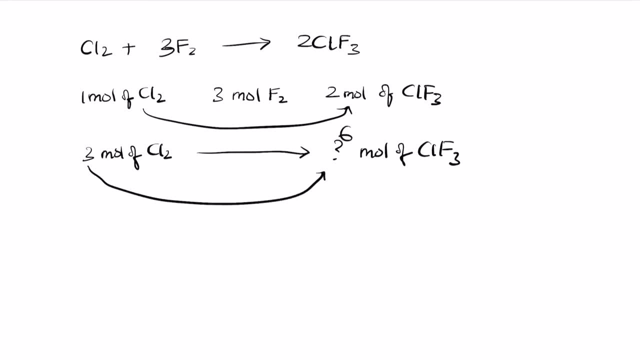 you should get a total of six. so remember one is to two. for each mole you are getting two of them, but if you use six moles of fluorine, you are gonna get how much? so for three you generally get two, which means that for six you 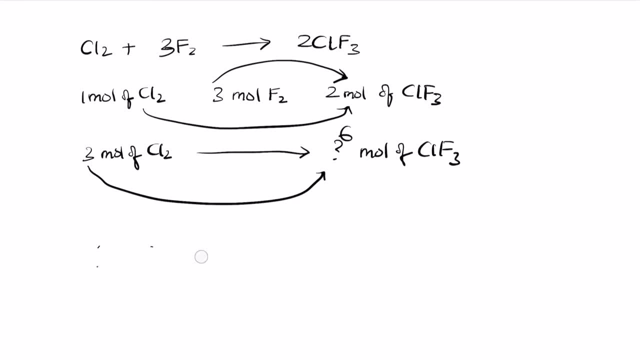 have to get. so let me write it down here, a separate part. so for three moles of fluorine, you get two moles of clf3. so for six moles of chlorine, what is the amount that you end up with? so let's consider the x. so 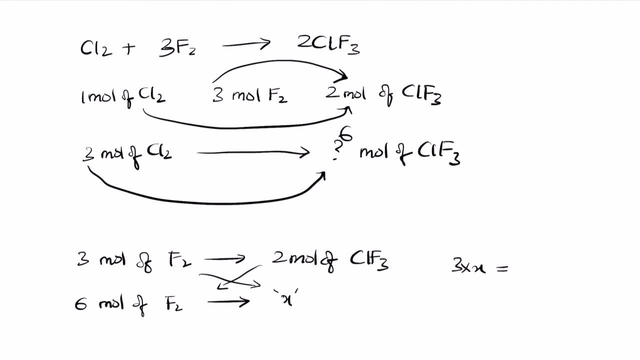 cross. multiply the value, so you get three times x is equal to two times six, so x becomes two times six by three. so three ones, three, twos, four moles of, so clf3. so when you use three moles of chlorine, the answer that you are getting is six moles of clf3. 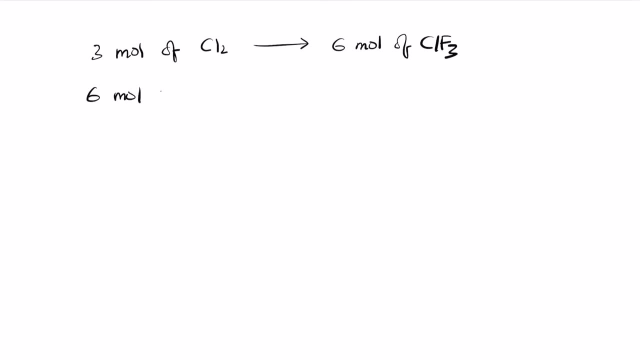 but when you use six moles of fluorine, the answer that you are getting is four moles of clf3. the reactant that gives you the smallest amount of product is the limiting reactant. so reactant that gives you the smallest amount of product limiting reactant is the limiting: the one that gives you the smallest amount of product. 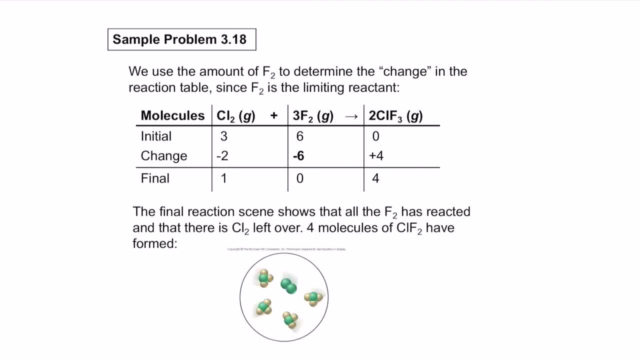 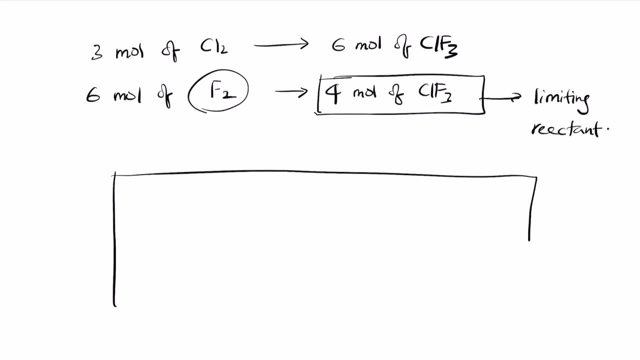 in comparison is the limiting reactant. so now, how do you write it in the reaction table? is we start by using a small table? so let's start by using a small table. and how to write down the reaction sensor. so we start on the top by writing down the reaction. 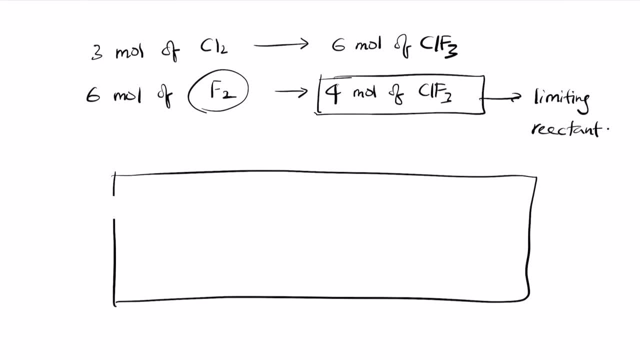 the reaction, not the reaction in the one, not the actual balance reaction. so this is the molecules. so the reaction is cl2 gas plus 3f2 gas gives clf3 to clf3 gas. so the first one we want to write what is the initial amount? 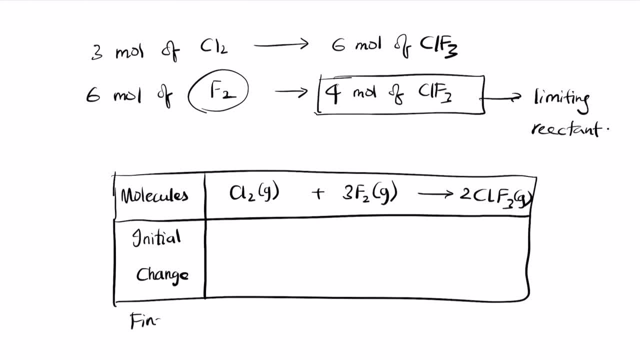 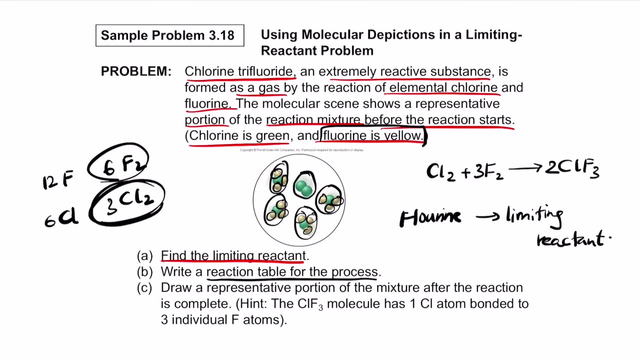 what is the change that is happening and what is the final amount left? so how do you write this reaction here? so initially we had three molecules of chlorine, so write down the three molecules of chlorine. and we had a total of six molecules of chlorine in the reaction, so six molecules of chlorine. 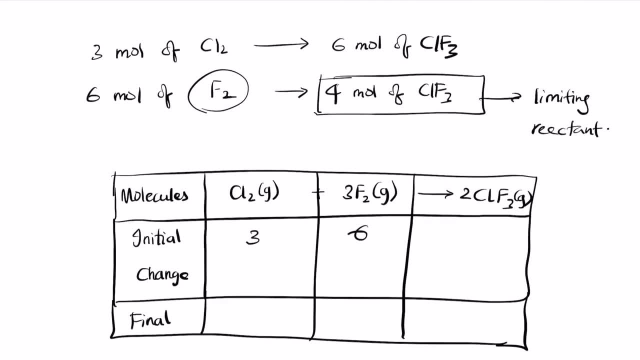 and we have three. so there were four of them. so there were zero initially, because nothing happened in the reaction in terms of the change. how many molecules are utilized here if you look at the actual reaction? so there is four of them that are going to end up forming now. how many fluorine are? 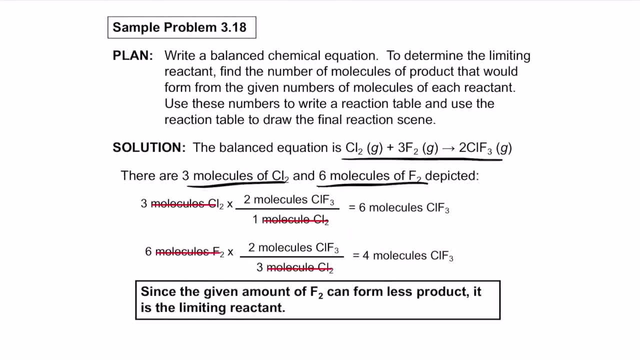 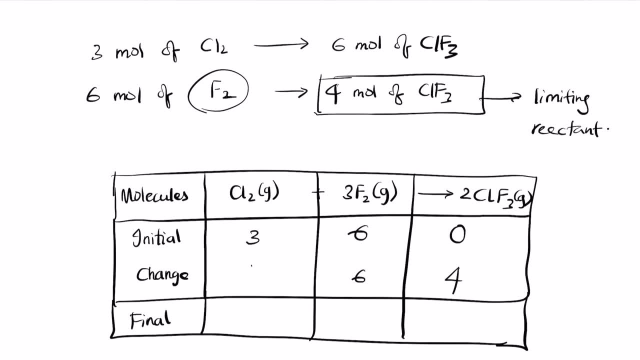 being utilized completely here. so there is four. four of them are completely used. all six of them are completely utilized. but there is one chlorine left, so that one chlorine is the final one. that's left right. so it means that here there is four and here there is zero. so what is the change in the number of chlorine? is there is only minus. 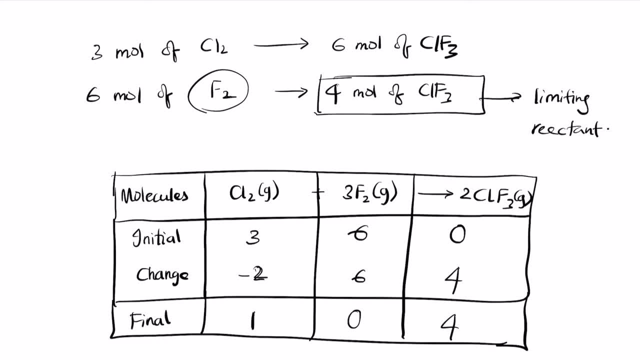 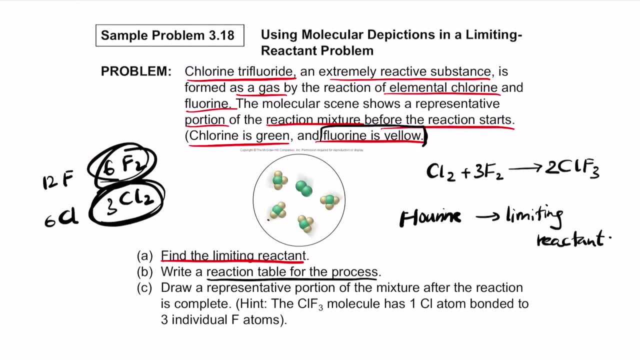 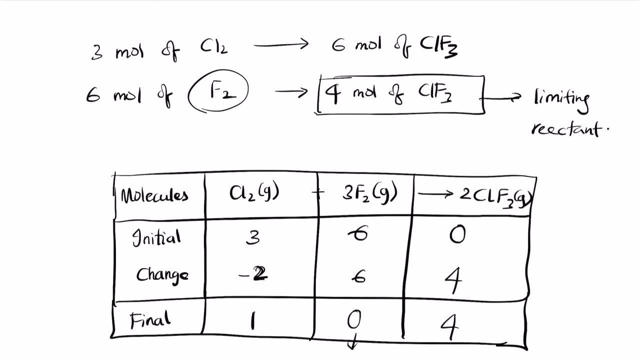 two. so only two of them are being utilized in total and there is one left, so notice the one here. so this is the one chlorine that's left in the reaction. so whichever one is completely utilized, this is the limiting react. so amazing. whichever one becomes zero in the reactant side in the reaction table, this becomes the limiting. 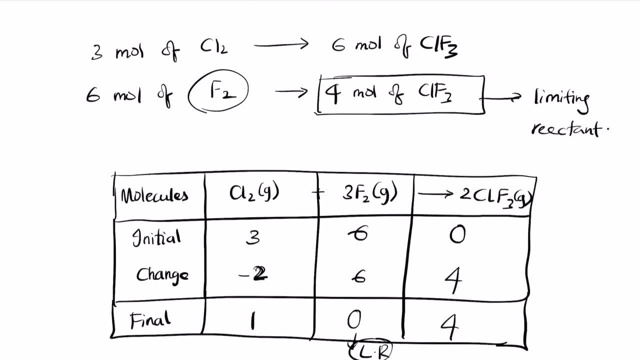 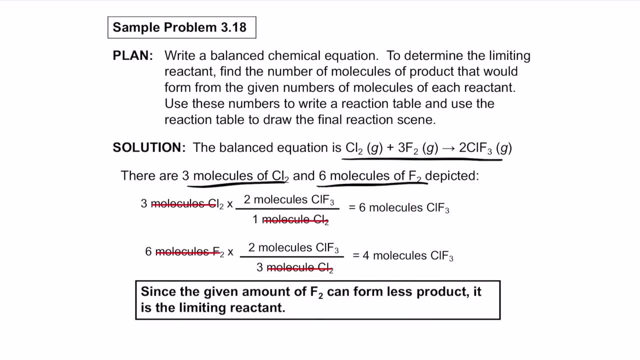 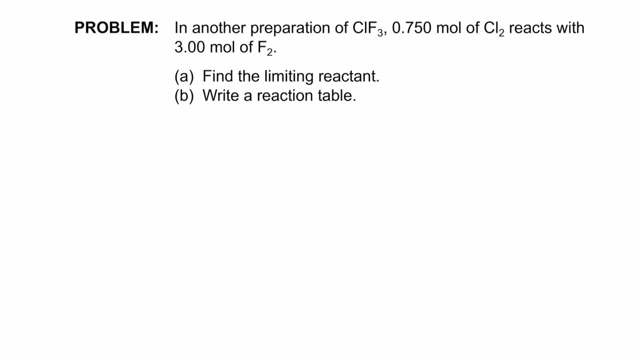 reactant. so we will learn more about this as we go along, but this is the simplest version of how to calculate the limiting reactants. so let's take an example, let's take another example of this and let's try to find how to use the reaction table to find the limiting reactant. so now this: 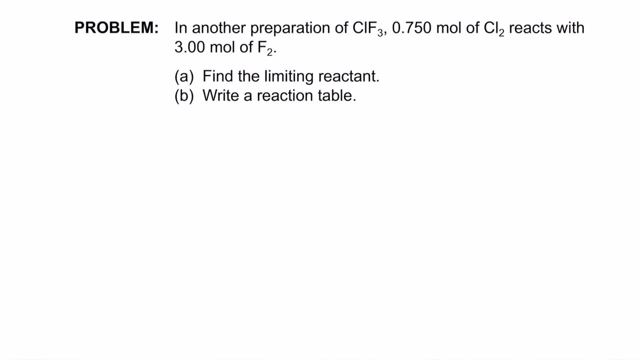 is the same problem. again, we are using different moles of each quantities. now first thing is write down the balanced equation. so the balanced equation is: cl2 plus 3f2 gives 2clf3. so which means for one mole of chlorine you get two moles of clf3 and for three moles of fluorine 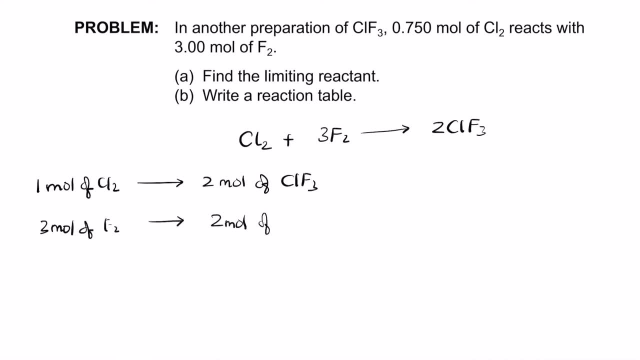 you get two moles of clf3. now in the first reaction they have given us 0.750 mole of cl2 and 3 moles of f2. so now use that to write down the actual values. now let me write this as a separate part, so that so in the reaction we are using 0.750. 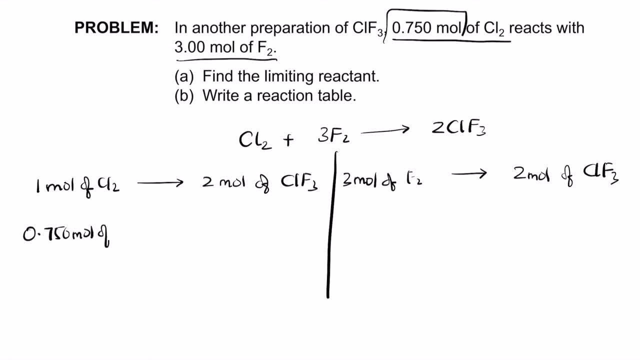 moles. so for 0.750 mole of cl2, what is the value that you get here? so again, cross multiply. so when you get 1 times x is equal to 0.750 times 2, so x becomes 1.5 mole. so this here is 1.5. 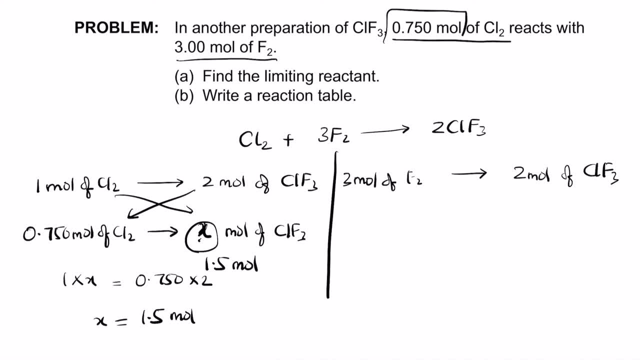 but notice the amount on the other side, which is 3 moles of f2 here, so they're asking 3 moles of f2 gives 2 moles of clf3, so they're again asking 3 moles of f2. so it's the same amount. so we don't. 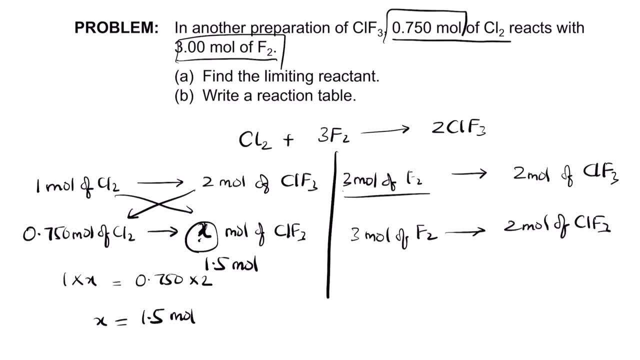 need to calculate also. so you get 2 moles of clf3 in one answer. you are getting 1.5 mole in one answer. you are getting 2 mole. now how to recognize this and write it down in the reaction table. so notice in total, what is the amount that you are using in total? 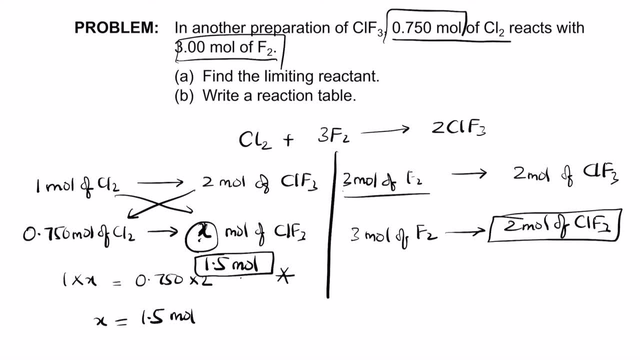 so in this, which is the least amount. so this is the least amount. now, forget the part that you get 2 for right and write down the 1.5 mole of clf3. remember that this is the actual product that forms, because this is the least amount. so what is the amount of chlorine that you utilize then? so for if 1.5, 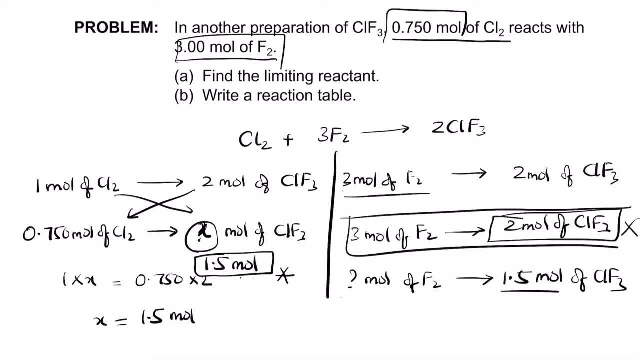 mole of clf3 is the product. what is the number of moles of chlorine? again, cross multiply. so 3 times 1.5 is equal to this is x. so x times 2. so x becomes 3 times 1.5 by 2. so that gives you a. 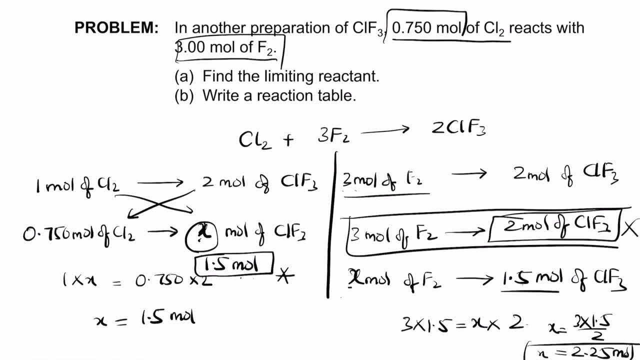 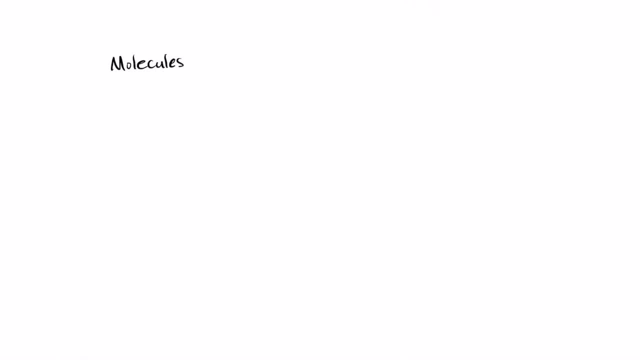 value of 2.25 mole. so this is the value that you end up with now write down the reaction table. so in the reaction table you have molecules, you have initial, you have the change. now you have cl2, cross, 3f2 forms 2, clf3. 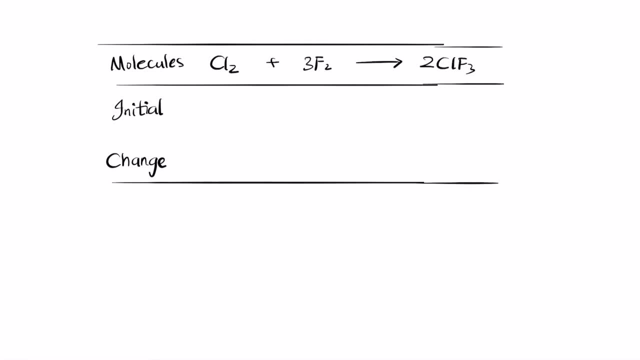 so initially there was how much chlorine in the reaction? 0.750 mole. 0.750 mole. and how much fluorine was there? 3 moles, so that is 3.00. so what is the limit of chlorine in the reaction? 0.750 mole. 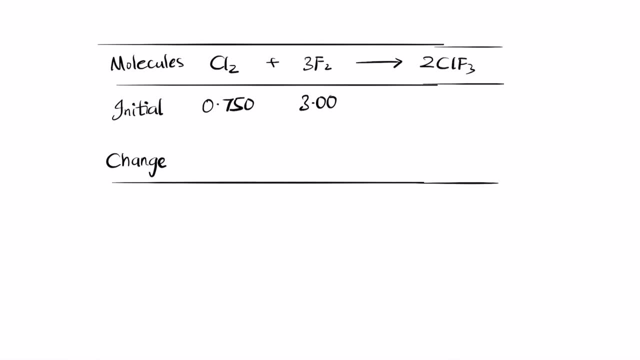 getting 3 or is limiting product that you get 1.5. so originally, initially, there is 0 because it is the product next. what has changed here? so we know that you end up getting 1.5, 0 Molar clf3, because that is the least amount that you can get now because which is the limiting? 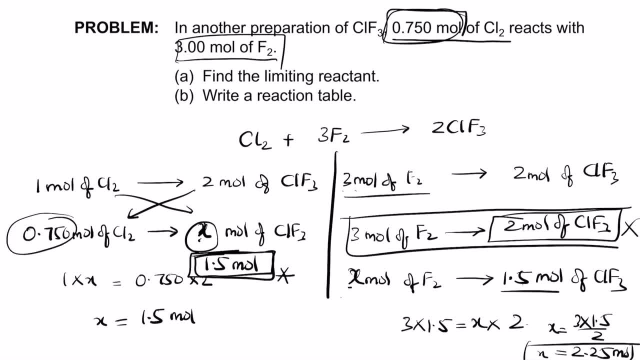 reagent here. so chlorine is the limiting reagent, so it utilizes completely, so it becomes 0.750. so which basically means that the final one will be 0. now we want to know how much chlorine are. there is 1.5, so what is that? 150 ml followers, so this is 1.5. 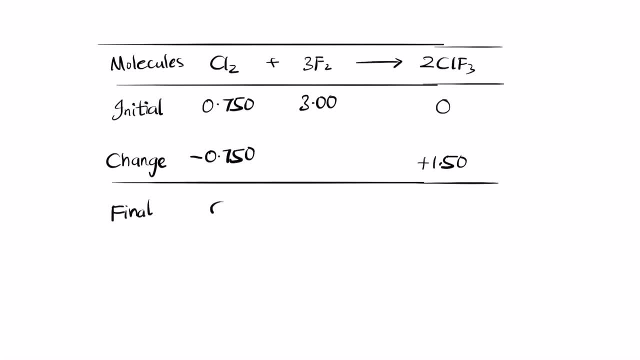 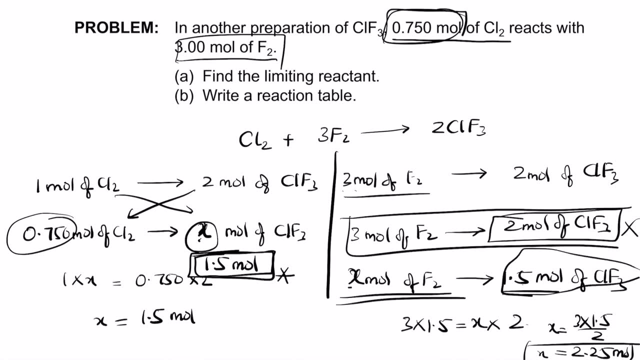 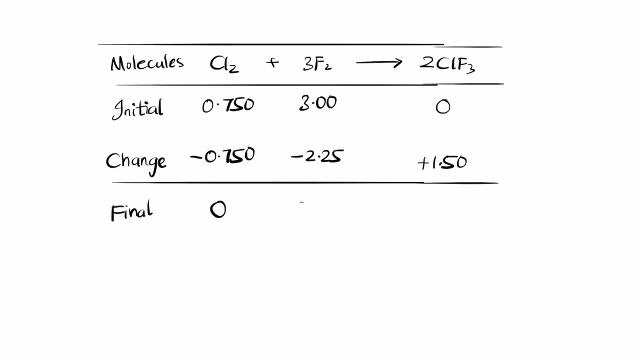 zero. so it basically means that the final one will be zero. now we want to know how much of the fluorine is utilized. so for 1.5 mole of clf3, we calculated what is the amount of fluorine. that is 2.25 mole, so it becomes negative 2.25. so the product that is left is 0.75. so for 1.5. 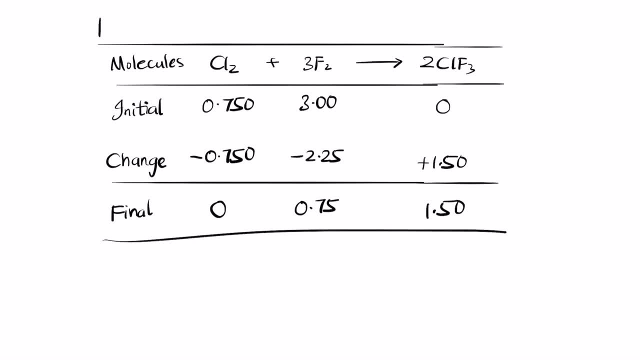 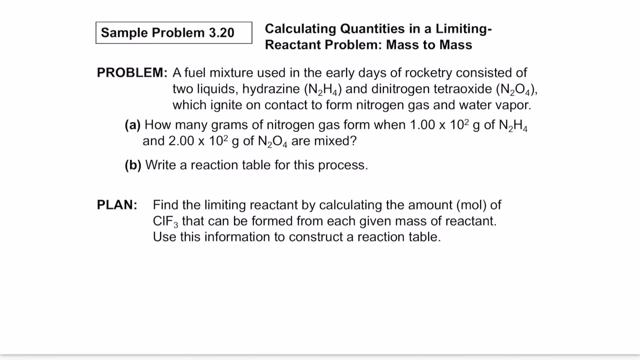 this. here is the reaction table, and in this reaction table we found that chlorine is the one with zero, which means this is the limiting reactant. so this is how you can draw reaction table for any given problem that involves the batteries. so now try this problem. here we have. 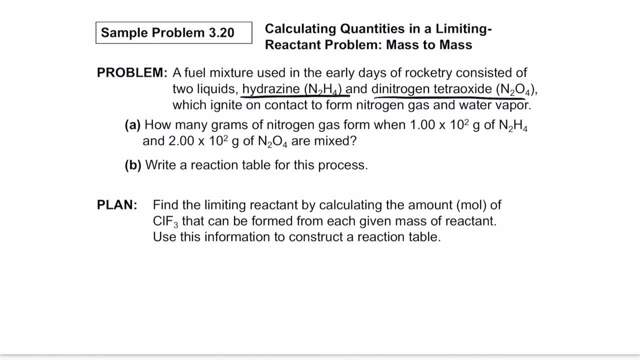 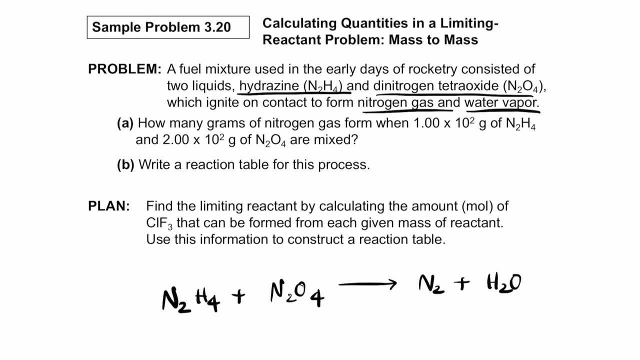 two liquids, hydrazine and dinitrogen tetroxide, which will ignite on contact to form nitrogen oxide and water vapor. so the reaction is n2, h4 plus n2. o4 gives n2 plus h2, so the balanced equation is 2 n2- h4. 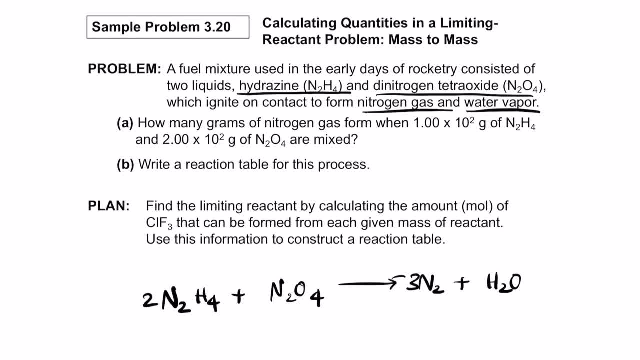 plus one becomes 3 n2 plus 4 h2. so this is the balance equation. so remember the values are given in grams. so first convert the mass into the number of moles, so by using the n formula, m by m, and then catry using the reaction table and try to write down the values. so it's similar to the last. 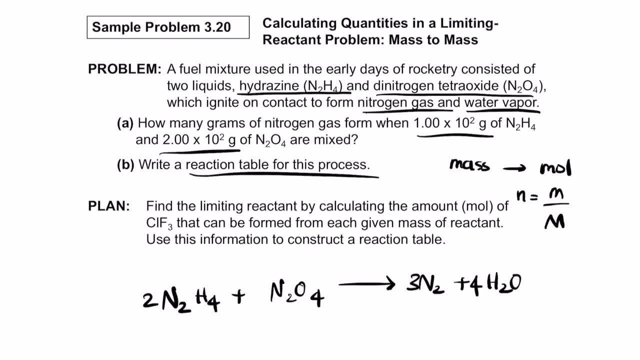 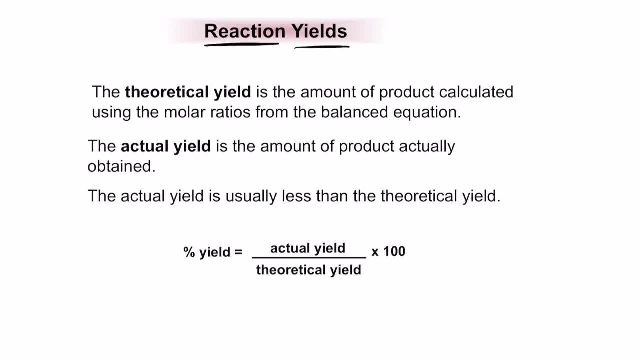 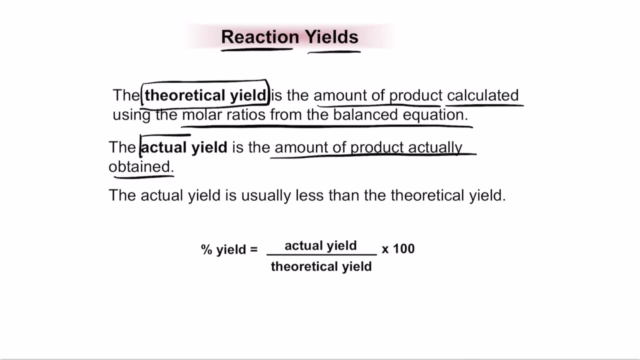 problem. so pause the video right here and try to solve this problem. so next is the topic of reaction. so what we generally get- the amount of product that can be calculated using the molar ratios from the balanced equation is called as the theoretical yield, but the amount of yield that you end up getting actually is called as the actual yield. 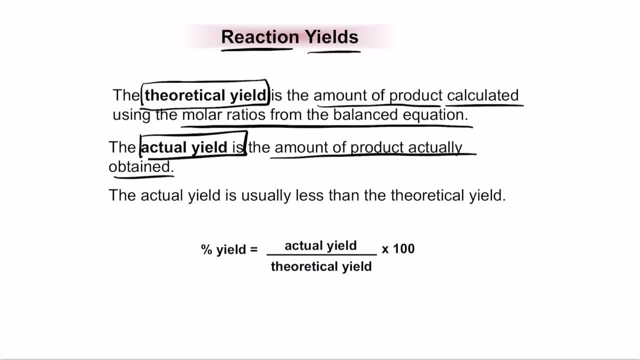 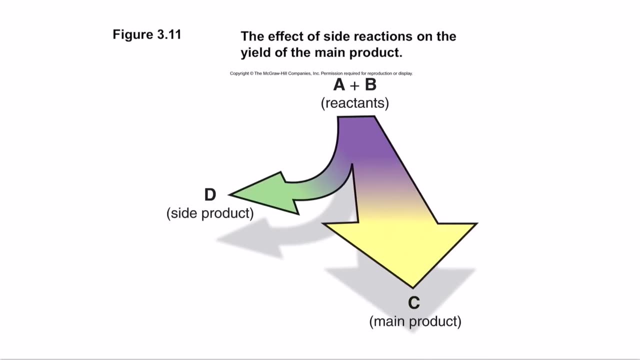 right. so the actual yield is usually generally less than the theoretical yield and it can be calculated by using the percentage yield. so percentage yield is the amount of yield that you get out of the theoretical yield. so that is actual yield over the theoretical yield times 100. so you're only going to get some part of the main product, so some of it. 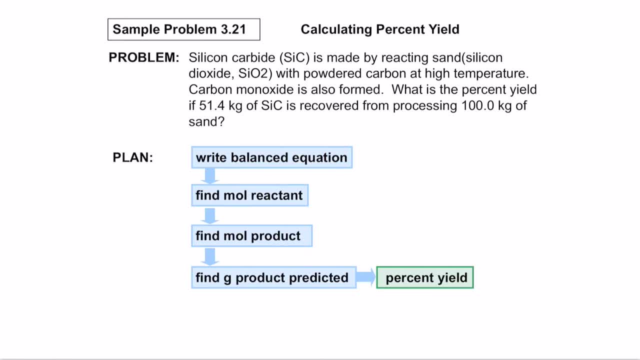 is going to end up being a byproduct. so let's take an example of this. so silicon carbide is made by reactant sand with powdered carbon at high temperatures, so and carbon monoxide is also formed. so what is the percent yield if 51.4 kilograms of silicon carbide is recovered from processing 100? 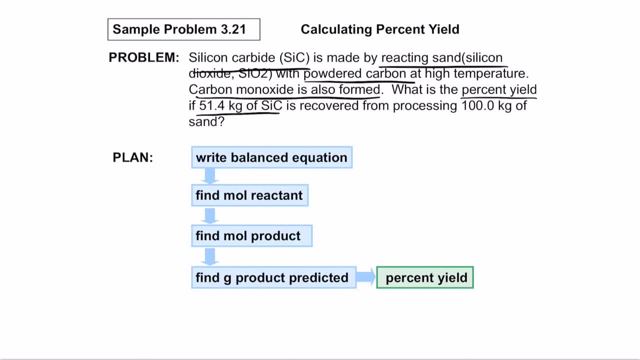 cages of sand. so remember that you have to write down the reaction first. so si o2 is reacted with carbon dioxide, so if you look at the reaction, it's already balanced, so you don't need to balance it more than that. notice that it has one carbon. so there is two carbons here, so write down two. 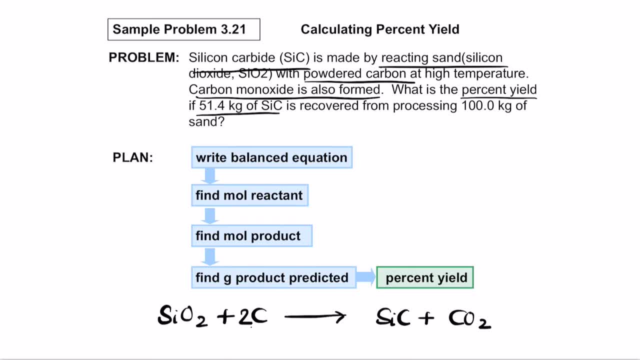 carbons. so si o2 plus two carbons becomes si c plus co2, so that ends up balancing the reaction. I'm sorry, it's carbon monoxide so, which means that si o2 plus there are two carbons on that side and there is only one oxygen being used, so you have to use two oxygens when you. 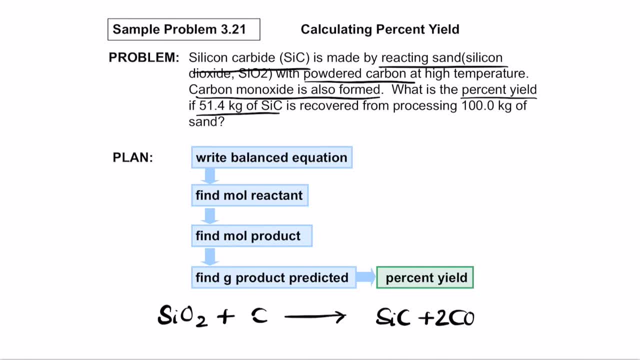 use two oxygens, it becomes three carbons. so this becomes three carbons. so you have si o2 plus three carbons gives si c plus 2c. so now, this is the balanced equation that you end up with. now let's take a look at how to calculate the actual yield. so the reaction is: 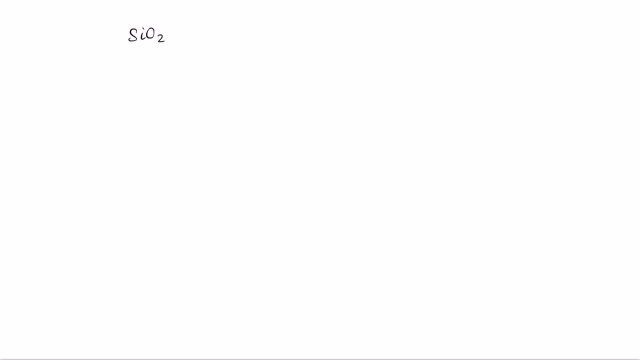 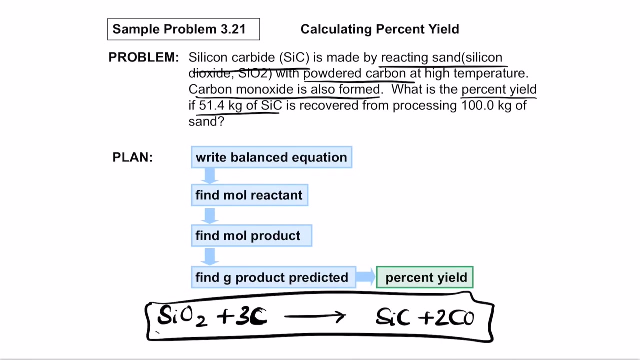 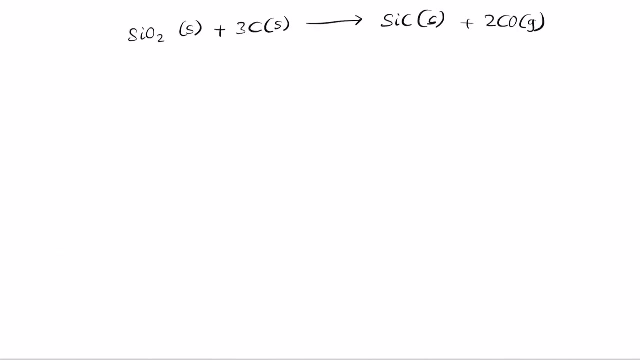 si o2 solid plus three. carbon solid gives si c solid plus 2 co, which is the gas now. in the reaction it said that what is the percentage yield if 51.4 kilograms of si c is recovered? so they have recovered 51.4 kilograms of si c, so what is the amount of silicon oxide? 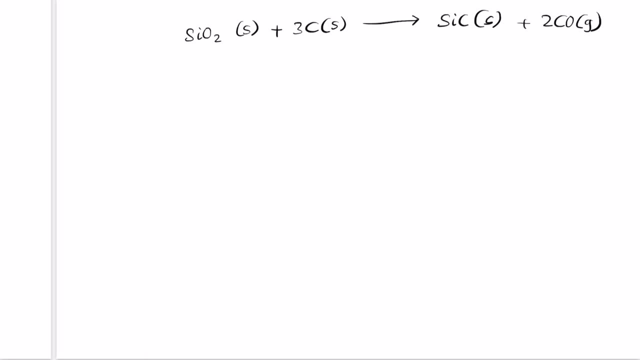 that is used. so when they are using here, they have used a hundred kilograms of sand. so this is 100 kilograms. so for one mole of si o2 I get one mole of silicon copper. so when you use 100 kilograms, remember that this is the mass of si o2 used. 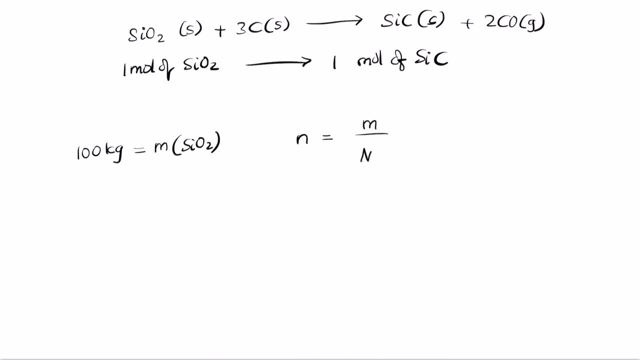 so we want to find the number of moles. so the number of moles is mass by molar mass. so mass is 100 kilograms into a thousand- remember that we need it in grams, so that is going to be 100 into a thousand grams. divided by the molar mass, so the molar mass of silicon carbide. so silicon has an 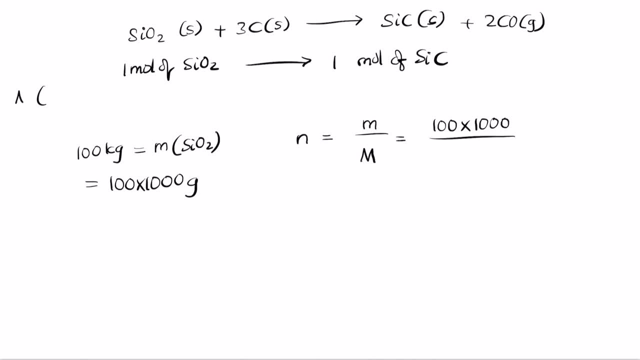 atomic. you know, molar mass silicon is twenty eight point zero nine and the molar mass of oxygen is sixteen point zero zero. so the value becomes 16 times two is thirty two plus you have twenty eight point zero nine. so the value is sixty point zero nine grams. 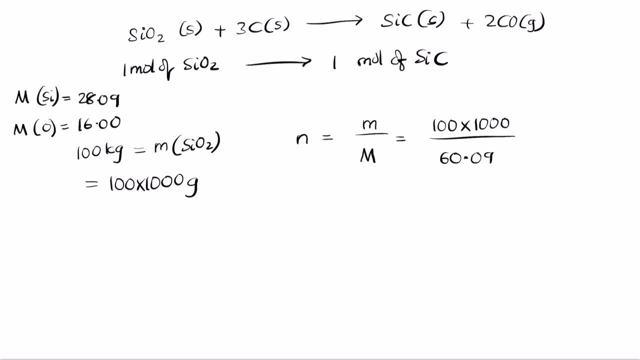 per mole. now calculate one hundred times one thousand over sixty point zero nine. so that gives you a value: one six six four point one six six four mole number that there is four maximum digits. so moles of si o2. so for one mole of si o2 you get one mole of silicon carbide. so if it is, 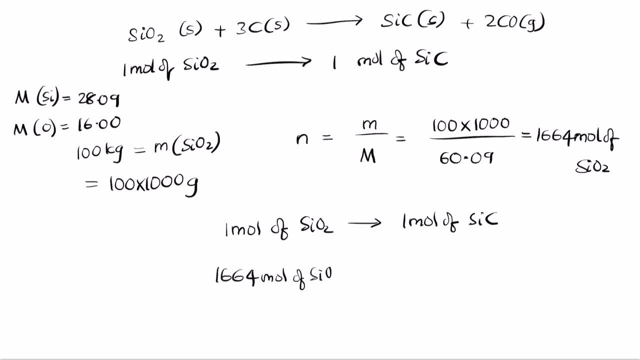 one, six, six four mole of si o2, and obviously one is to one ratio. so which means that you're going to get one, six, six four mole of silicon carbide. now, this is the amount of silicon carbide in mole, but we want to know its mass. so mass is number of moles into 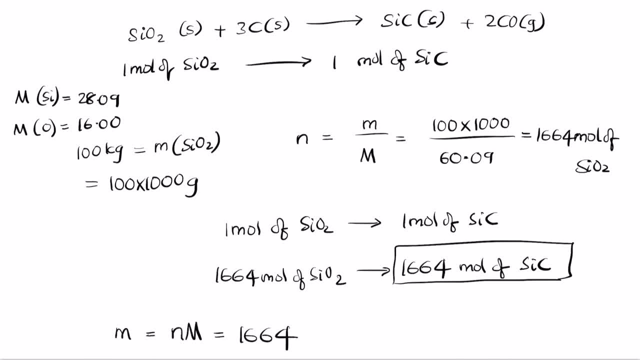 the molar mass, the number of moles is sixteen sixty four. we are remember that here we are finding the mass of silicon carbide, so sixteen sixty four times the molar mass of silicon carbide. so silicon is twenty eight point zero, nine. so twenty eight point zero, nine plus. 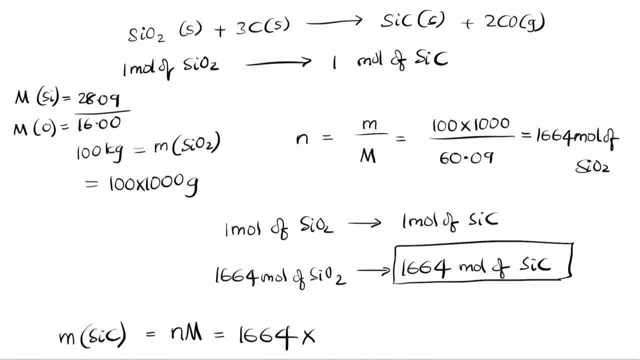 twelve point zero one. so that gives you a value of forty point zero. so the molar mass silicon carbide is 40.1. so when you you get the value of 667, 26.4 grams. so when you calculate it in kilograms, so 66.73 kilograms. so the mass of silicon carbide 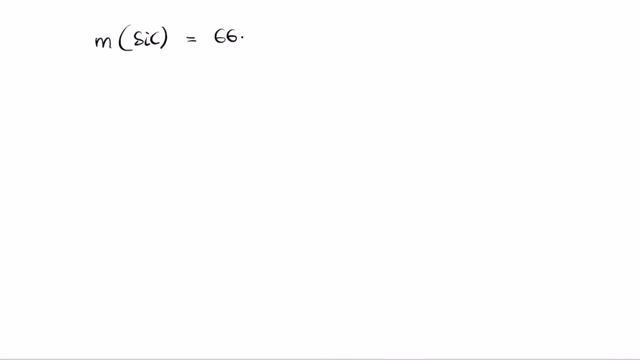 is 66.73 kilograms. so this here represents the theoretical yield. so this is the theoretical weight. but in the proper in the process you got 51.4 kilograms of silica cupid, so the actual yield is 51 point 4 kilograms. so when you want to calculate the percentage yield, so the percentage yield is: 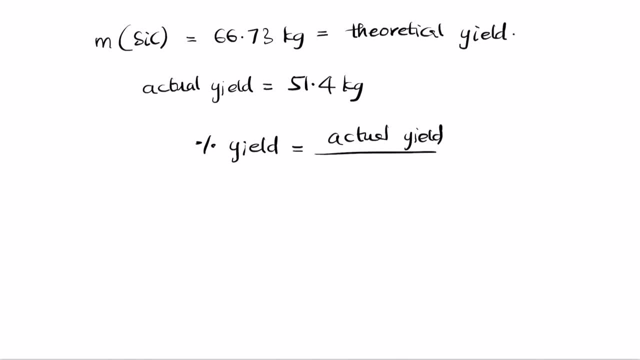 actual yield over the theoretical yield times 100. so the actual yield is 51.4 over 66.73 times 100. so when you calculate it you end up with a value of 77 percent. so this is the percentage yield. so which means for every 100 kilograms of sand, so for every 100 kilograms that you end up, 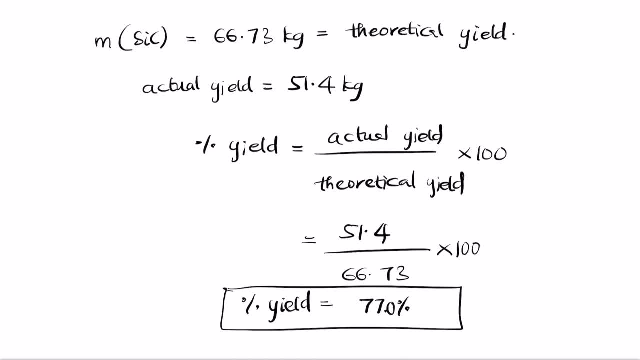 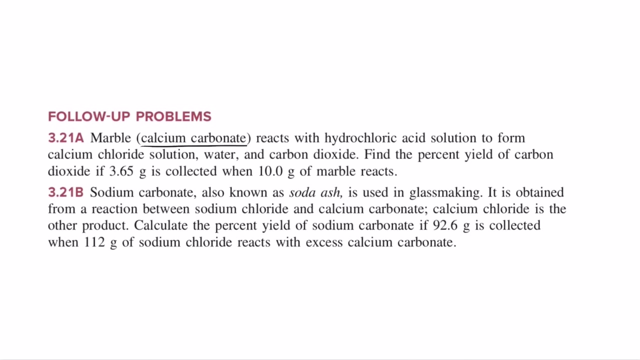 in theoretical yield, you only get 77 kilograms if it in actual yield. so this is how you can calculate the actual yield of any given reaction. so try these two problems. so here we have marble, which is calcium carbonate. reacts with hydrochloric acid to form calcium chloride and carbon dioxide, so calcium carbonate is. 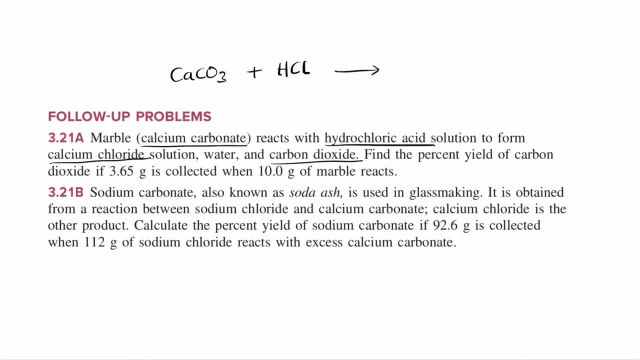 CaCO3 plus HCl forms CaCl2 plus H2O plus CO2. so so first balance the equation, next try to calculate the yield. here they have given that, find the percentage yield of carbon dioxide. so if 3.65 gram is collected, when 10 mal 10 grams, 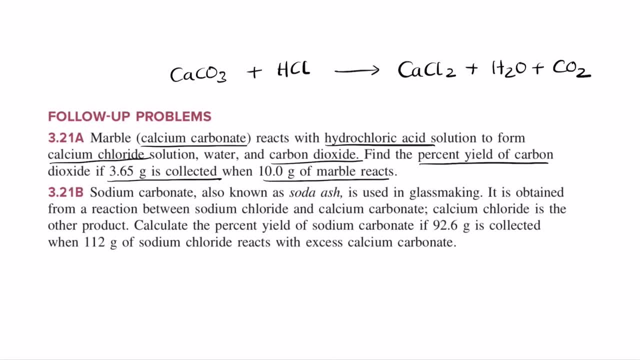 of marble reacts. so try this problem and see if you can get it. so try the other problem as well. also, try writing the equation on your own and see if you can solve the problem. so with that we end the chapter on stoichiometry. so